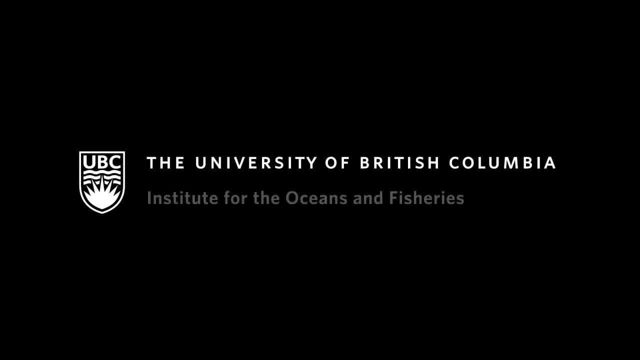 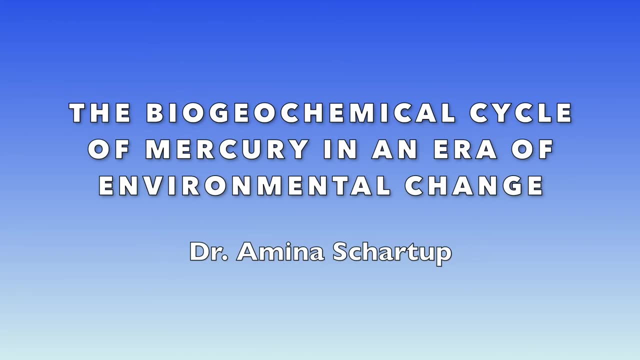 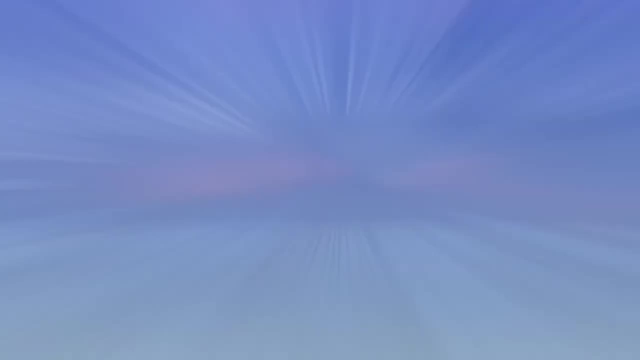 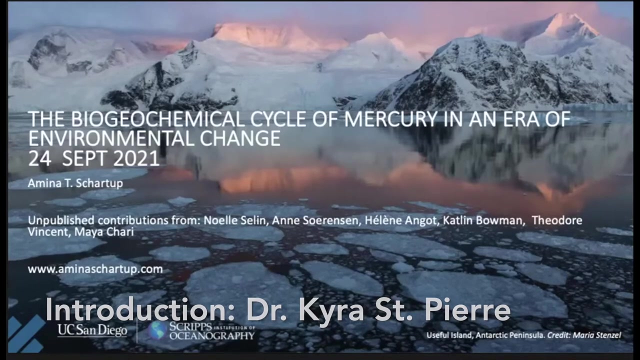 Great. So my name is Kira St Pierre And, for those of you that don't know me, I'm a postdoctoral fellow at the Institute for Oceans and Fisheries, And so today I'm thrilled to introduce Dr Amina Shartup as our presenter. When I saw kind of the call for speakers, 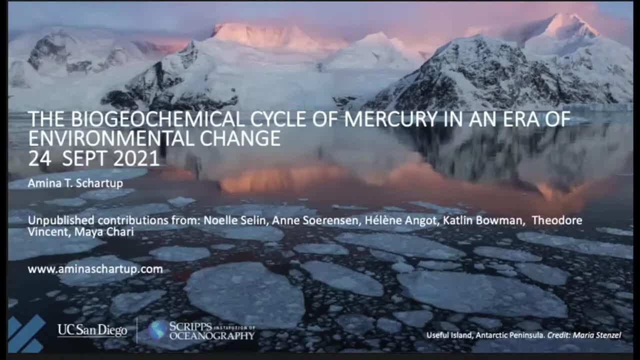 one of the kind of major themes for the UN Ocean Decade was this clean ocean, where sources of pollution are identified and removed, And so Dr Shartup fits amazingly in that theme, And that was one of the reasons that I suggested her for the seminar series this year. Dr Shartup is an 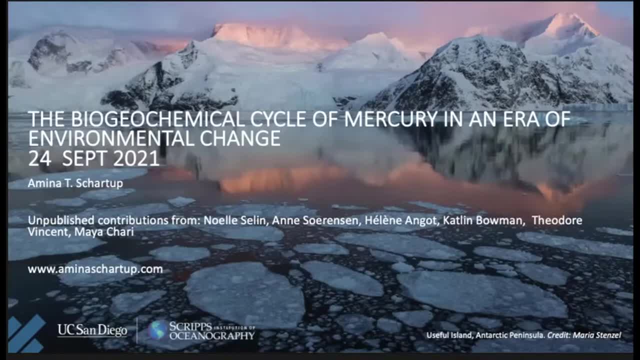 assistant professor at the Scripps Institute of Oceanography in California. She holds a PhD in oceanography from the University of Connecticut, a master's in science in geochemistry from the Institut de Physique du Club de Paris and a bachelor of science in chemistry from Paris. 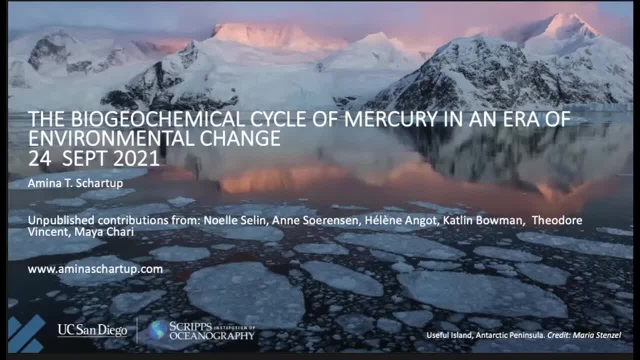 Descartes University, So she's a true interdisciplinarian. Before coming to Scripps, Dr Shartup was a research associate at the Harvard School of Public Health and the Harvard School of Engineering and Applied Sciences. She also spent two years as an American Association for 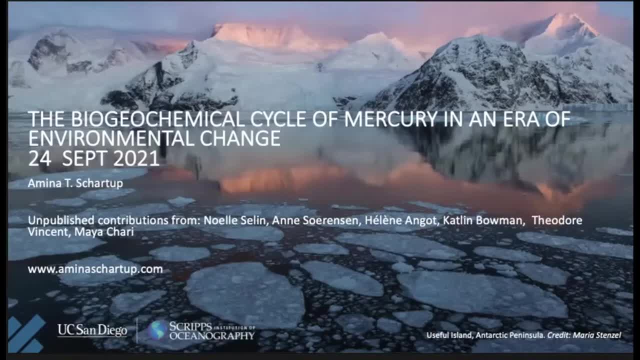 the Advancement of Science, Science and Technology Policy Fellow at the National Science Foundation's Office of Polar Program Arctic Section, during which time she developed a federal guidance document on pursuing ethical research in the Arctic. Dr Shartup's experience, both in 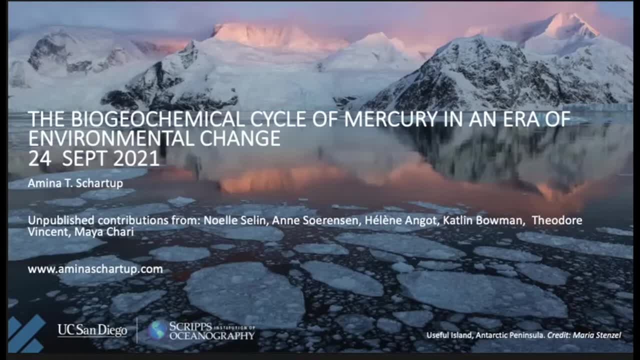 biogeochemistry and in policy has really put her at the forefront of research on neurotoxic methyl mercury in the world's oceans, covering everything from kind of very small scale biogeochemical speciation and bioavailability of mercury in aquatic environments to large scale ecosystem. 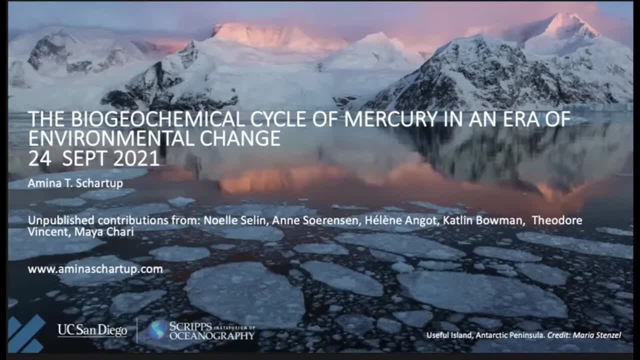 models tracing the effects of climate change and fisheries on the bioaccumulation of methyl mercury through marine food webs, some of which I'm sure she'll cover here today. So thank you for accepting the invitation, Dr Shartup, and I'll leave it with you. 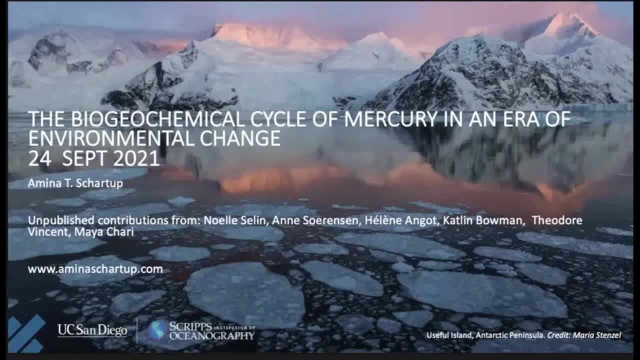 Thank you, Kira, for this fantastic introduction. I'm very flattered and really excited to be here today. I've seen a lot of amazing work coming from your institution that overlapped with some of my own interests, so it's really a great honor to be here. So before I kind 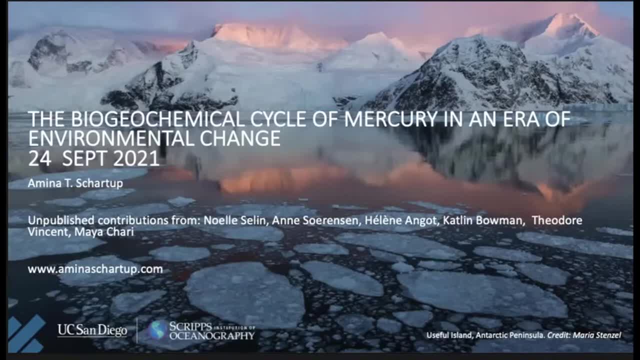 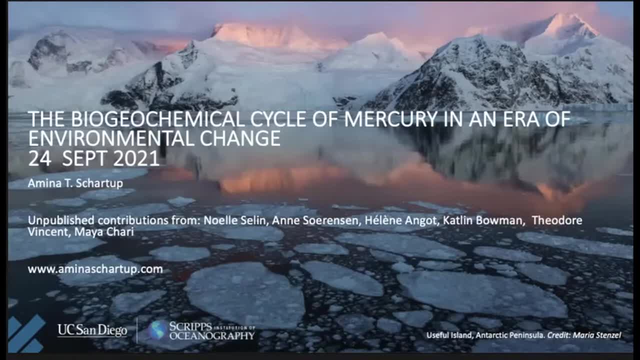 So I was born in USSA. So I was born in USSA. So I was born in USSA. that that's when I had my final slice. So after spending a few years in Baku, my mom and I moved. 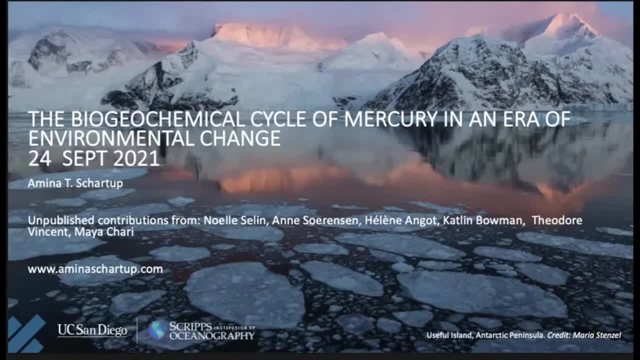 to West Africa, where my dad is from, And actually we moved to Mauritania more precisely, And I was told in school that Mauritania was one of the most bountiful seas in the world. They had a lot of fish, which now makes sense. It's an upwelling region, So indeed there's a lot of productivity. 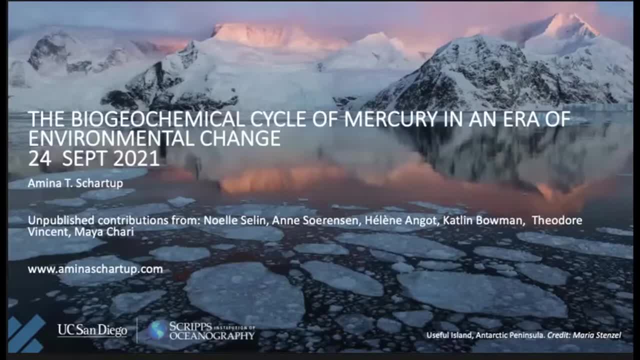 And it was a fantastic place to grow up And we actually lived in the neighborhood that was nicknamed Little Russia And it's a funny story. I actually learned how to write in Russian when I moved to Mauritania, Because when I left the Soviet Union I was six, So I couldn't really 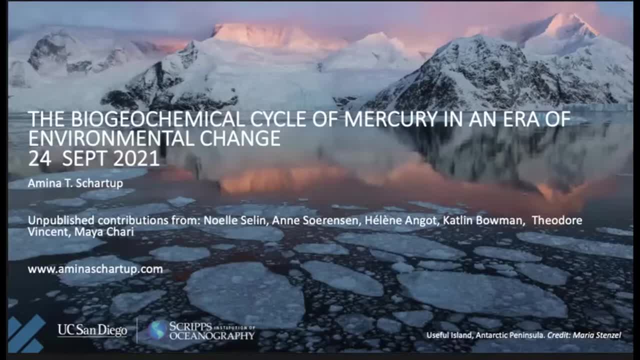 write really well, But I learned there because there's a lot of like a big Russian community And so there were many of us who are mixed race children, we spoke Russian, run around the desert and so on, And the reason why there's such a big Russian community in Mauritania was because right after 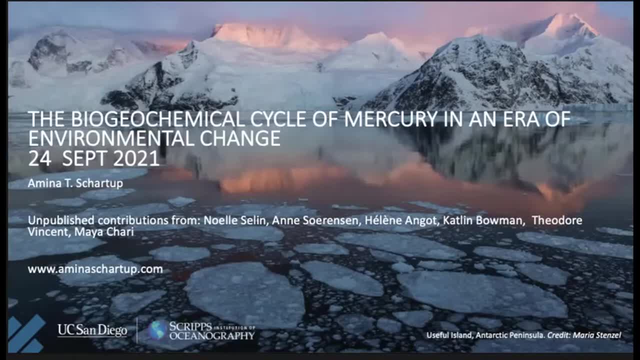 independence from France, the Mauritania struck a deal with the USSR to in exchange for access to fisheries, they would send their- mostly sons- to get educated in USSR, And so that's how come a lot of them went out there and they occasionally brought children to the USSR, And so that's how come a lot of them went out there and they occasionally brought children to the USSR, And so that's how come a lot of them went out there, and they occasionally brought Russian wife, And so that's why there were many of us mixed race children. So of course it didn't. 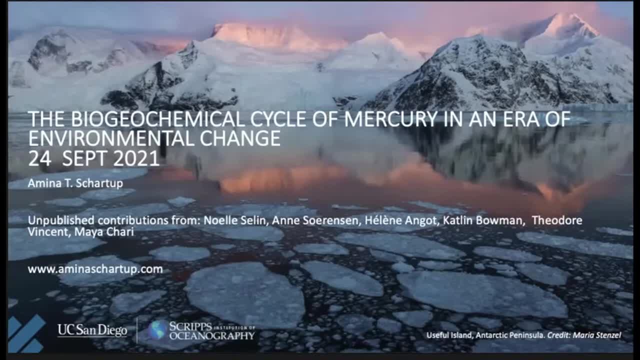 take very long before we started hearing of over exploitation of the coast and small local fishermen having to go farther and farther out to be able to collect the fish that they needed for subsistence living. So it was kind of funny to think about it, both at a time and later on, how the socio economics 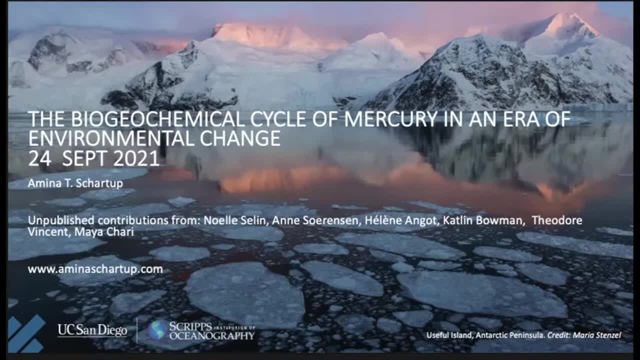 developed, but also the cross-cultural environment And and and my and the fisheries and my own existence right. because had they were not, if they were not sending those people to get educated in USSR, We wouldn't exist, right. so it was kind of like a funny thing to think about. 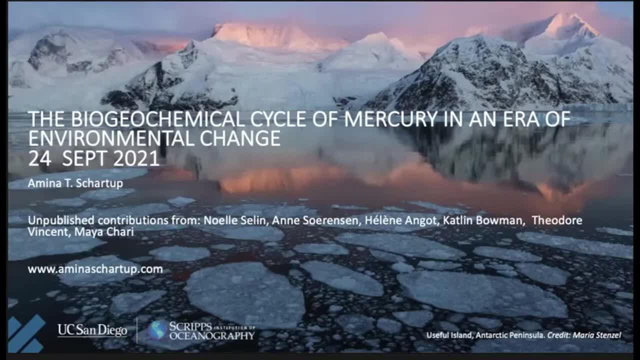 Those environmental issues, but in the context of society and my own contribution to those issues. Anyway, Long story short. I'm interested in the Murphy's Cycle but it's mostly driven to the future, driven to the fact that I'm interested in how human behavior and environment in the decision 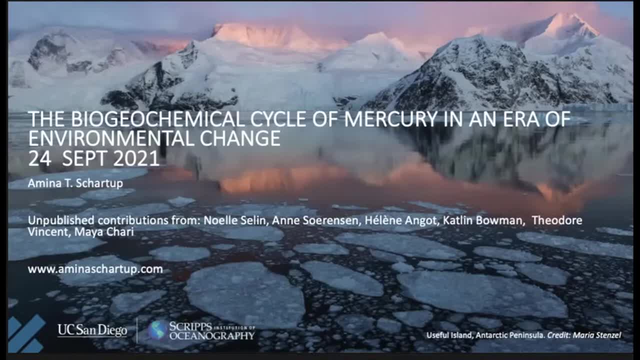 making process it really connects it and really understanding the science, but not really without putting in the broader context of what it means for society and human health. Most of the work that I'll be talking today has been published, so I'm not listing here the authors, but there has been some unpublished contributions that I will mention, and so 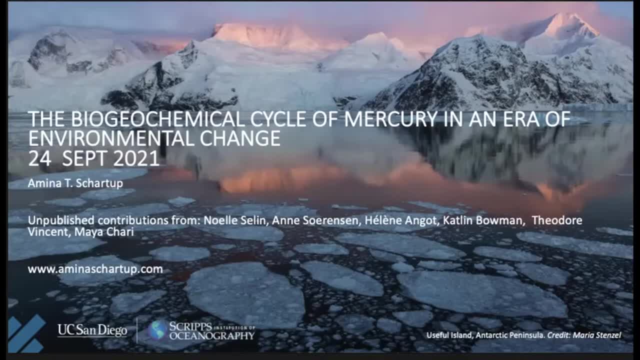 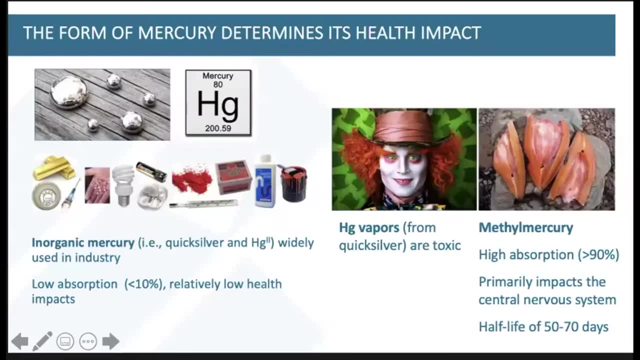 the authors here are Noelle Sleen, Anne-Hélène Angot, Kathleen Bowman, Theodore Vincent and Maya Charridos- last two actually my students. So for those of you who don't know, I'll give you a brief introduction of the mercury cycle and then we'll move on to talking about some of the projects that. 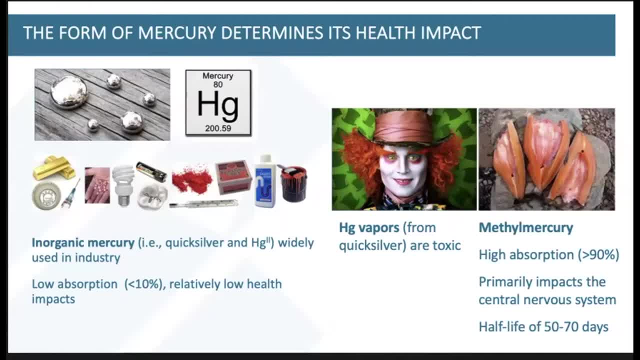 I've been working on, mostly in a chronological order. I find mercury really fascinating because it ties this, like I said, the industry, environmental change, earth, biogeochemical cycles, but also has this whole human history, community and individual health component to it. 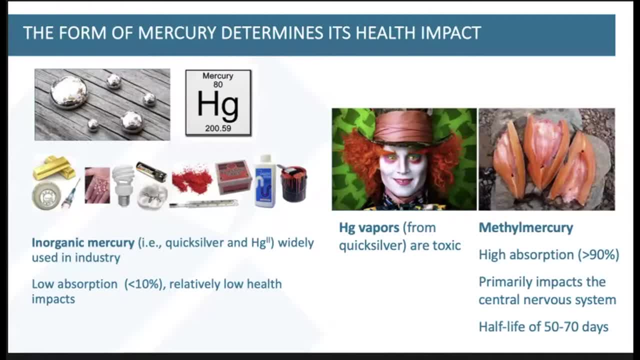 Mercury is about 3,000 years of use in its mineral form in this bright red pigment that has been found in Egyptian tombs and ancient Chinese pottery. But as many elements of the mercury cycle have changed over the years, there's a lot of work to be done on this, So I'm going to give you a brief introduction of the mercury cycle. 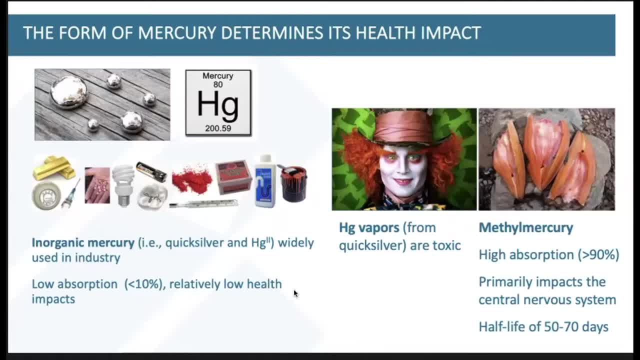 So here we have some of the elements we've been working on. this is mercury. this is mercury. you can see here some elements and as many contaminants or usages. in general, they substantially increase since the industrial revolution and now mercury has been widely used. 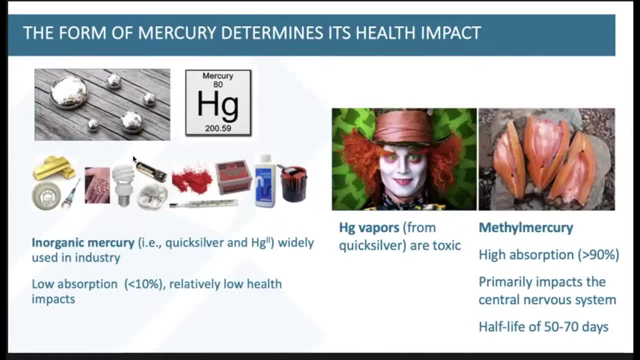 in industry and you may have heard of mercury usage in gold mining. Those CFL light bulbs have mercury. a lot of UV bulbs have Mercury, so there's like a really wide breadth of industrial use. mercury that you find in most of these products is actually not that toxic because it has a low 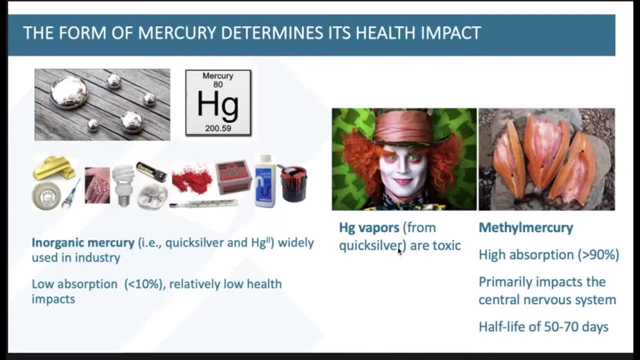 absorption rate in organisms. However, mercury vapors- you may have heard of the use in the felting industry and what it did to neurological health of the workers- as well as organic forms of mercury, methylmercury, which is actually the one that people refer to when they speak about. 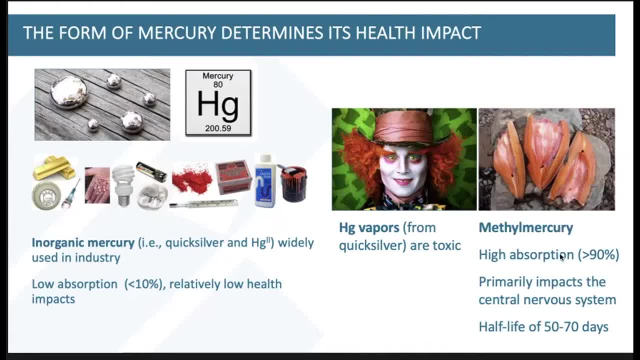 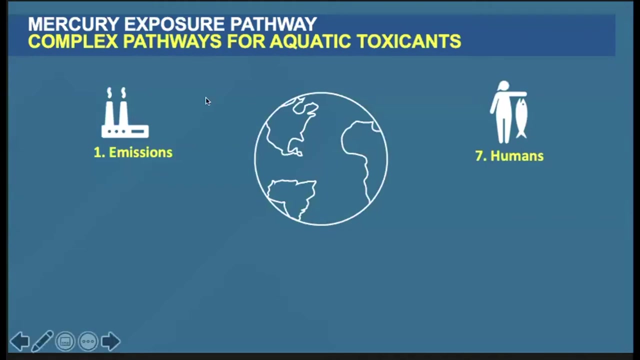 mercury in fish is actually talking about that organic form of mercury. It has a high absorption efficiency in biological tissues and it primarily impacts the central nervous system. so any higher level animal that has a central nervous system is particularly at risk. Fortunately for us, mercury is emitted into the environment through 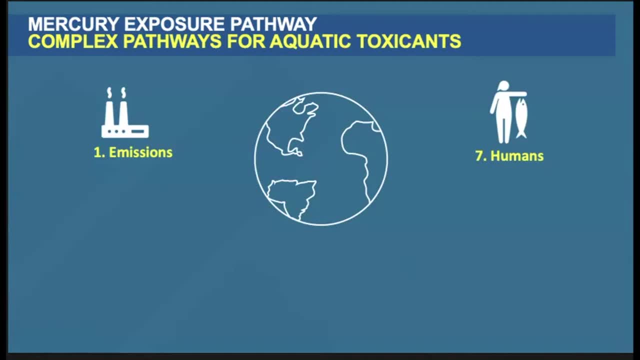 those industrial activities, with coal burning and artisanal gold mining being some of the biggest sources, and it ends up in fish and it impacts humans through consumption of fish for the most part. However, the system is complex and it doesn't go directly from emissions to 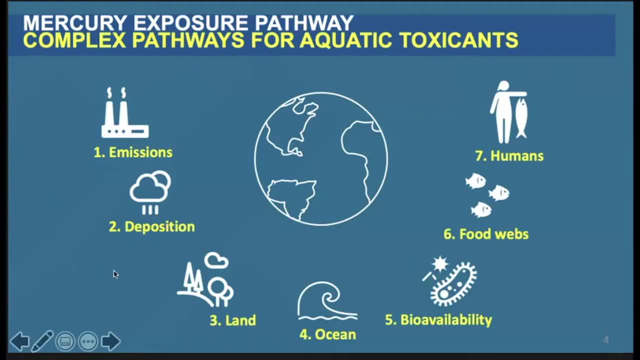 consumption by humans. It goes through a range of processes in the atmosphere, deposits on land, it cycles in the ocean, it is transformed microbially in the environment and then it enters the food web. where then food web processes and dynamics impacts this ultimate exposure? 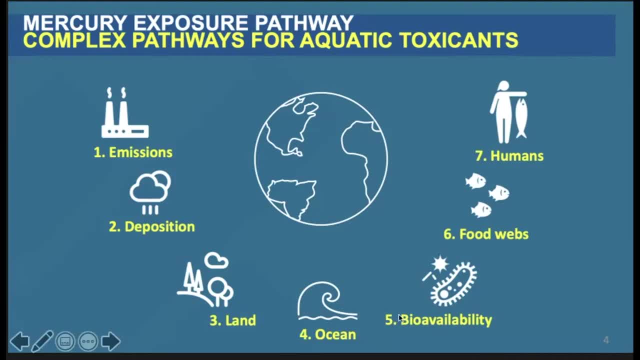 So, as you can see, at every step of the way here there are additional levels of complexity because these are interaction with the environment that we all know is changing. So I'm interested in actually almost all of the aspect of the mercury cycle and of how it has worked on some aspect in most of these steps. 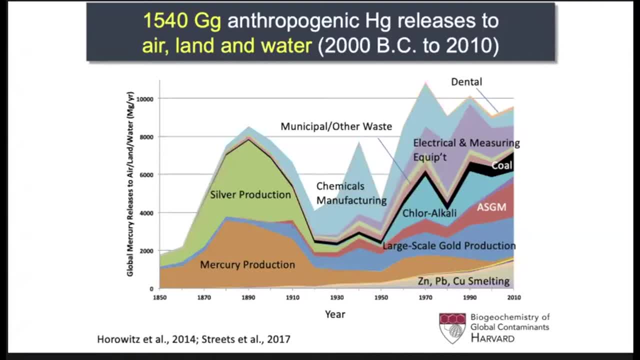 Another level of complexity in the mercury cycle is that the usages and emission and releases have changed over time. So you can see here- this is work by Hannah Horowitz- looking at global releases and emissions of mercury since 1850s And, as you can see, as we approach today, the complexity. 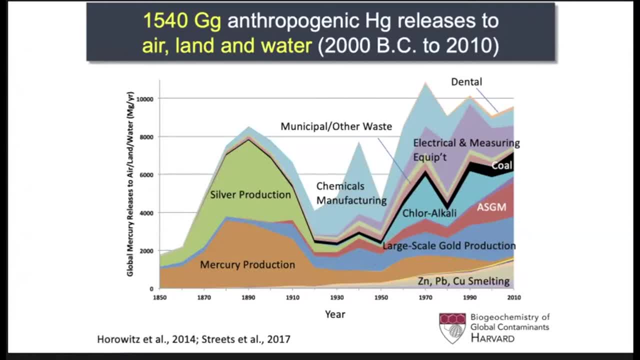 of the sources of mercury to the environment have increased, And so of course that type of complexity also comes with the fact that controls are becoming more difficult because there are different sources of mercury. But let's say we manage to get this under control and reduce releases of mercury into. 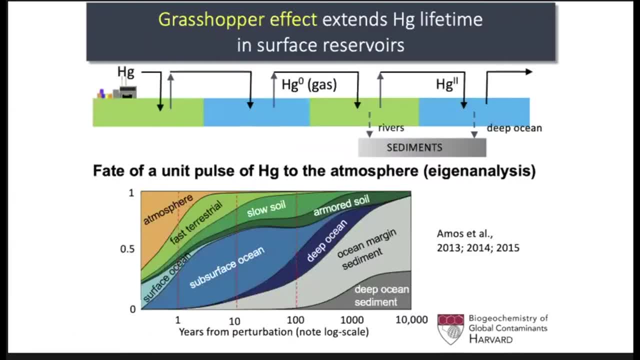 the environment we're also running into. an additional little problem is that mercury has this grasshopper behavior where, once it's emitted, deposits, it has a redox cycle that allows it to be re-emitted, So it kind of bounces around the environment and takes a little while to then be buried in the sediment. 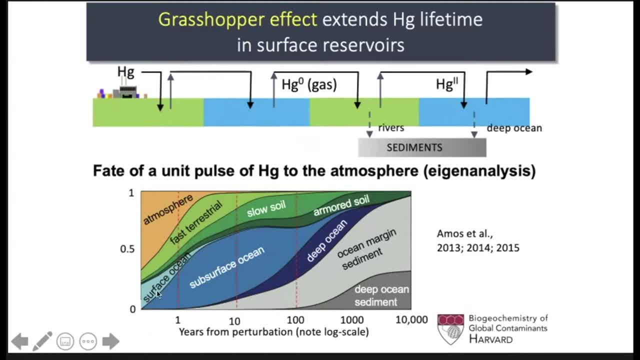 So Helen Amos did some work trying to replicate this through a model, and she replicated this effect of releasing mercury into the atmosphere and then tried to see how long it takes before it's buried and enters the geological cycle. And so at this time, zero, here she emits. 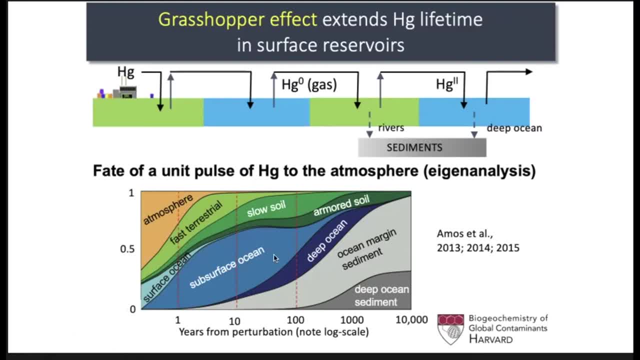 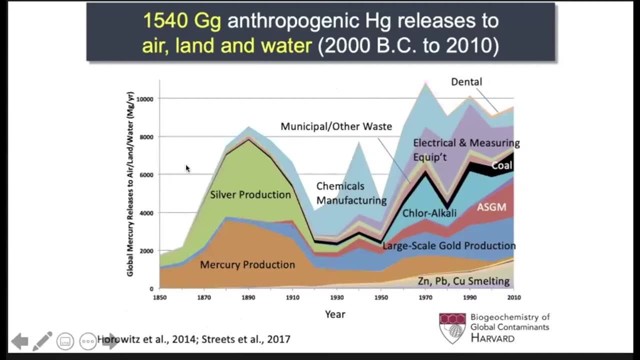 mercury into the atmosphere and then, as you can see, it takes a hundred to a thousand years for it to to start getting buried in those sediments, Which means that that mercury right there that we emitted a century or two ago is still cycling through the environment today. 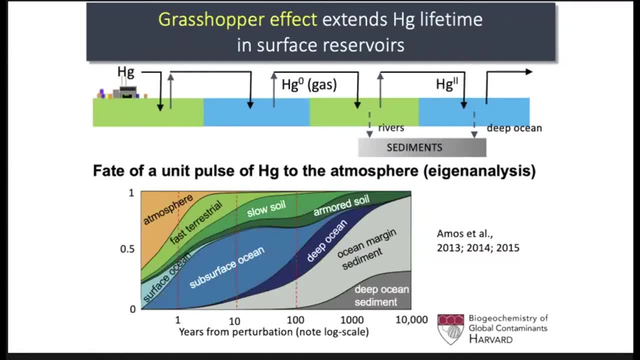 It also means that the mercury that we are releasing today is going to be cycling in the environment for the next hundred or so years. That means that we are going to have an overlap between those environmental and global changes that we're observing and the mercury that we are releasing today. So we estimate about two thousand tons. 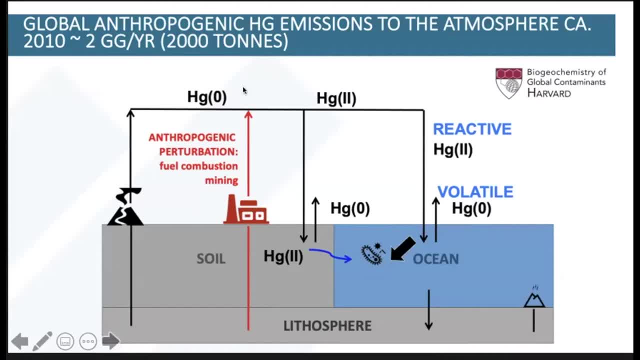 of mercury a year are emitted through anthropogenic activity. This mercury then has this, like I said, grasshopper effect when he bounces around before he reaches the ocean. Once it reaches the ocean, that's where it is transformed into the organic species of mercury, which is methylmercury, and then it biomagnetizes. 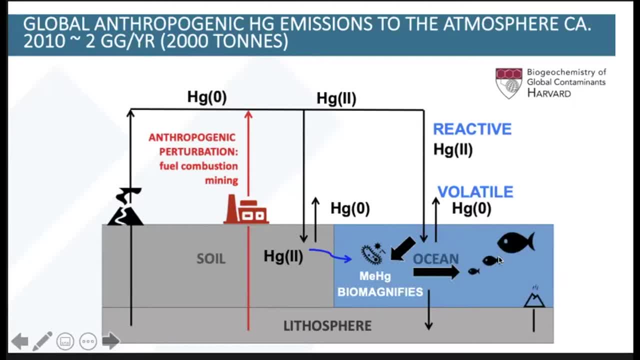 in the food web. So at every step of the of every trophic level, the concentration increase and they tend to reach fairly high concentration at the top of the food web, particularly in high trophic level. predatory migratory fish species such as tunas. 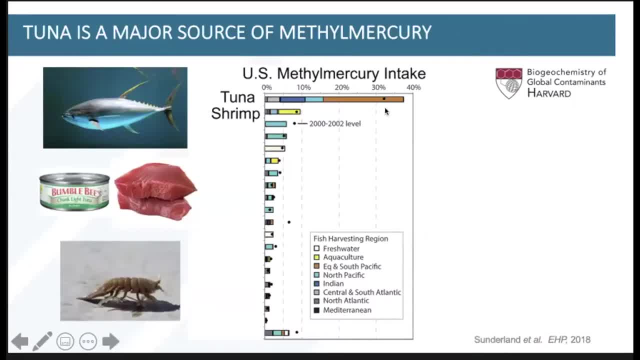 And tunas end up as a result, because people like to eat them and they have mercury, high mercury levels being a major source of methylmercury exposure. This is an example for exposures in the United States, where tuna is pretty much almost half of all the US methylmercury intake. 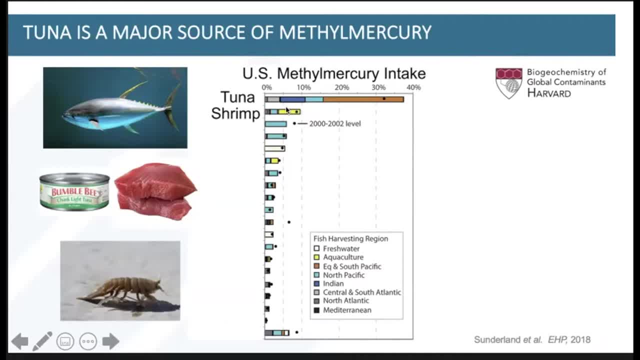 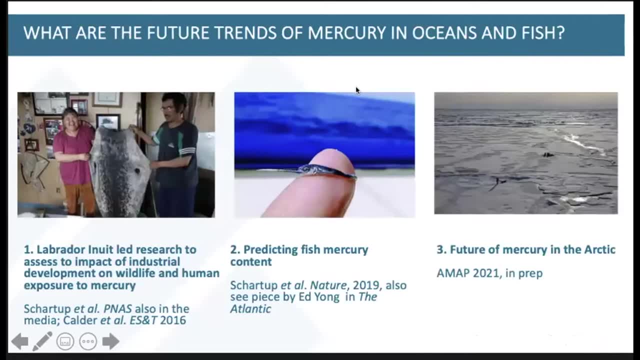 Shrimps come second. they're not particularly high, but people eat a lot of shrimp, so that makes up for it. So I'll walk you through a few examples of some work that we've been doing: working looking at the impact of industrial development following hydroelectric reservoirs. 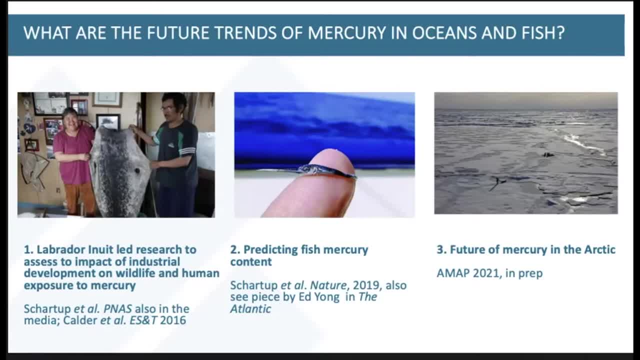 Creation and human exposure to mercury for the community living around the system. Another example: predicting fish mercury content as a result of environmental change. And then, finally, I'll talk briefly about some of the work we're doing for the AMAP, chapter 8 report, that is. 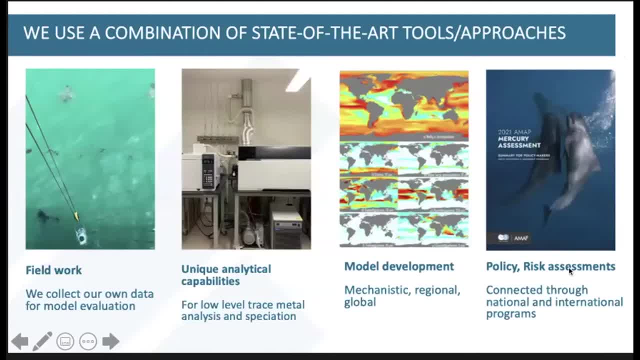 currently in prep In my group- in my previous group, we used a combination of different tools, So we do field work, So we often collect our own data that we can then use in model evaluation, And so it's kind of, in a way, allows us to develop models. 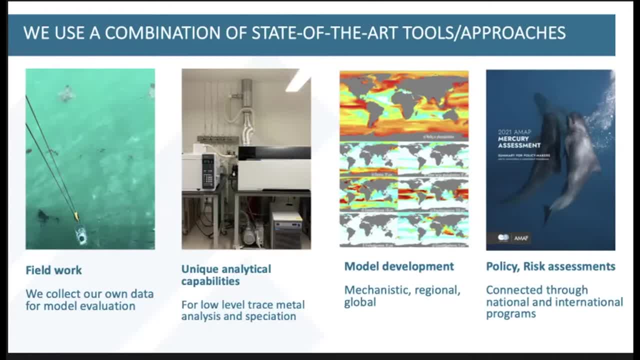 realize where are the gaps in terms of evaluating model data and be able to collect the data that is directly relevant for model development, rather than trying to gather from other work data. It can be somewhat mismatched in terms of timing, So we use our in-house analytical capabilities to do the work with a set of really low trace level. 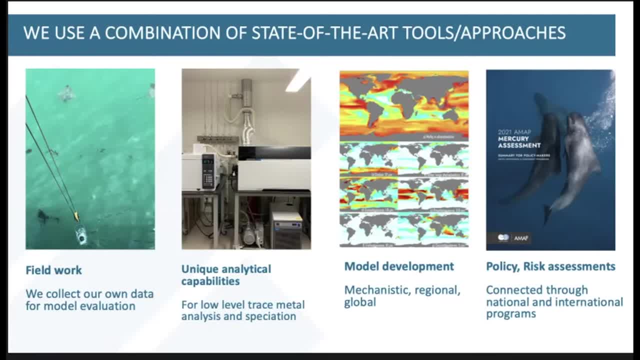 specialized instrumentation. We work on model development, as I've mentioned, both on the regional as well as a global scale, and we remain connected with the policy. as well as doing some risk assessment work allows us to connect to what are the needs on the ground in terms of 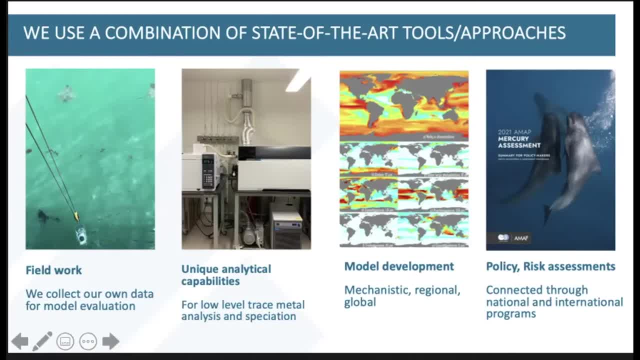 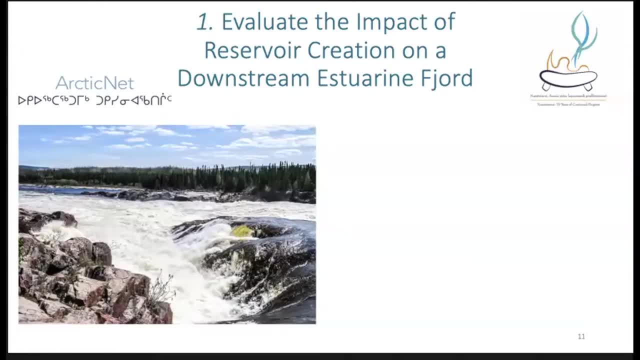 policy as well, as I'm looking for the word. forgot the word, sorry, it happens sometimes. So, example number one: we're looking at evaluating the impact of reservoir creation on a downstream fjord, and this was really driven by the Nazi government. 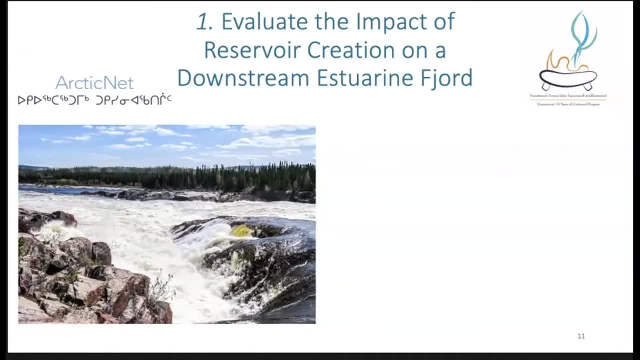 interest in trying to understand what is the impact of a planned hydroelectric development on three communities around the downstream environment of Lake Melville. It was driven by their understanding that of previous cases of exposure by indigenous communities living near reservoirs due to an increase in methylmercury in Canada. 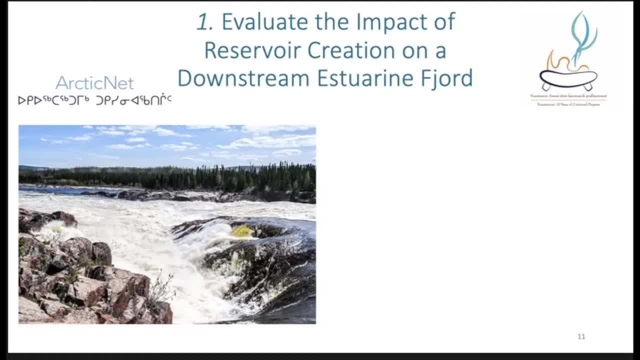 as well as in Brazil, following the development of reservoirs, And the reason for that is because, as I said, mercury gets emitted and then deposits into the soils. Most of the time, it's not just in the soil, it's in the soil, it's in the soil. 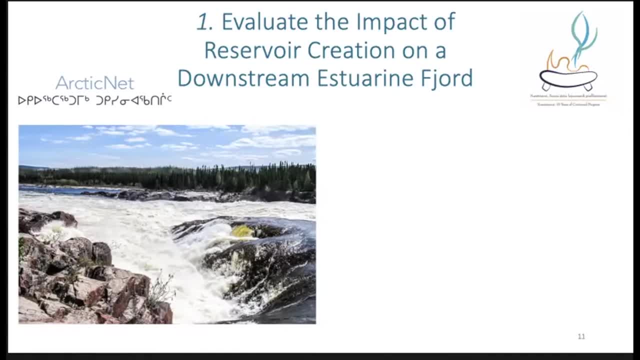 most of the time, when it deposits in soils, it doesn't really do much, just sits there bound to organic matter or other minerals. But once you flood that area, when you create a reservoir, you create the right conditions for the microbes that are living in there to transform that. 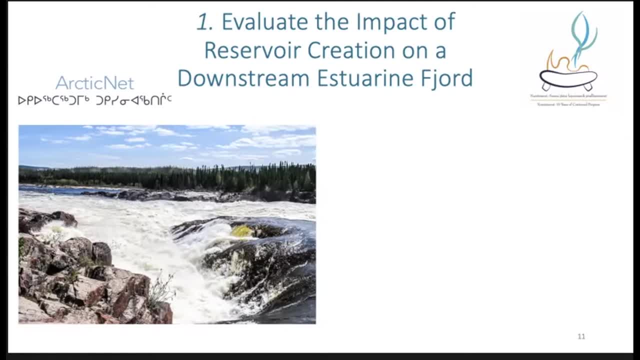 inorganic mercury that was just sitting there into methylmercury And there's a long history of well-documented cases of substantial increase in methylmercury levels in those freshly filled reservoirs and the communities living around the reservoirs that rely on the fish that 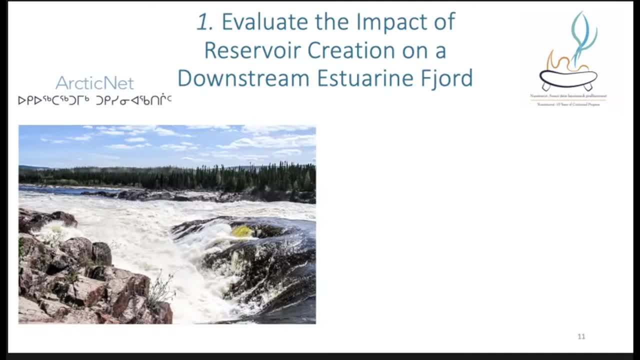 lives there being exposed to extremely high levels of methylmercury. So in that context, they were interested in finding out whether these impacts of increased methylmercury production will be seen downstream, in a downstream environment, from the reservoir. So this is the system. It's. 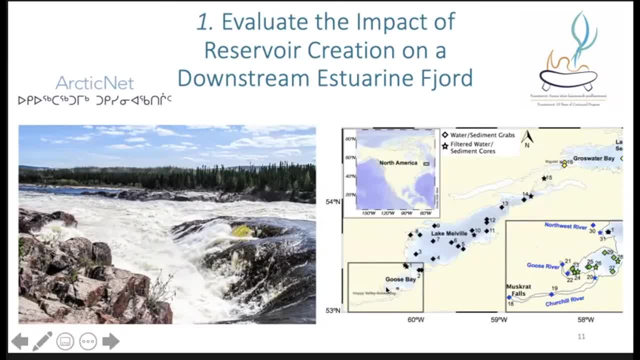 Lake Melville. It's not a lake, It's an estuarine fjord And the reservoir is planned right there in Musgrave Falls, which is about here, And the downstream environment is where we have several communities living here: Happy Valley, Goose Bay, Northwest River and then Rigolette, with Rigolette being 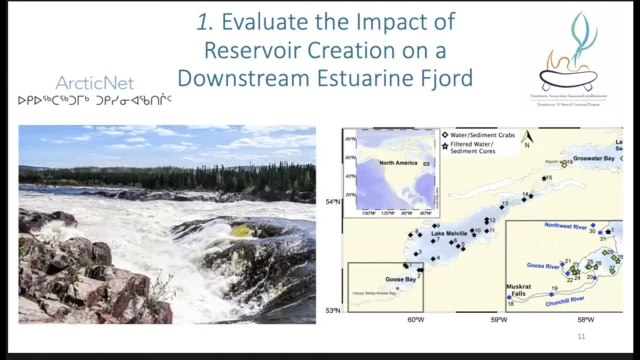 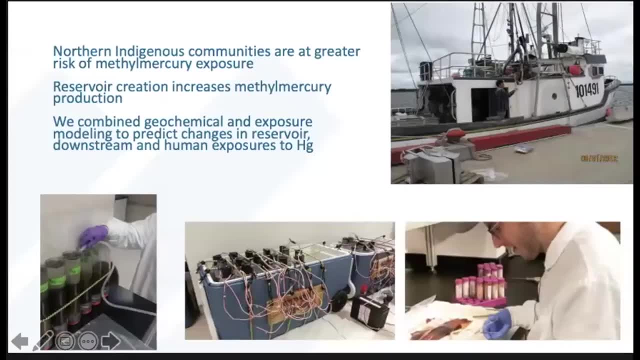 the community that is the most reliant on fishing and hunting around the system, And so what we were trying to do in this particular case is that we needed to link both the human community and the fish community, And so what we were trying to do in this particular 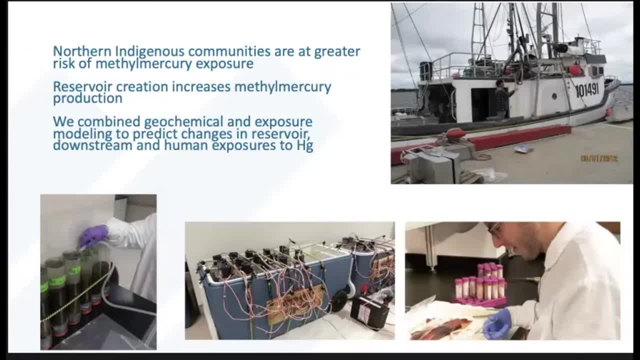 case was to take the geochemical component as well as the geochemical component and try to have some prediction, some ways to predict what the trends are going to be following industrial development. So there were like three parts to this One. we needed to understand the baseline. 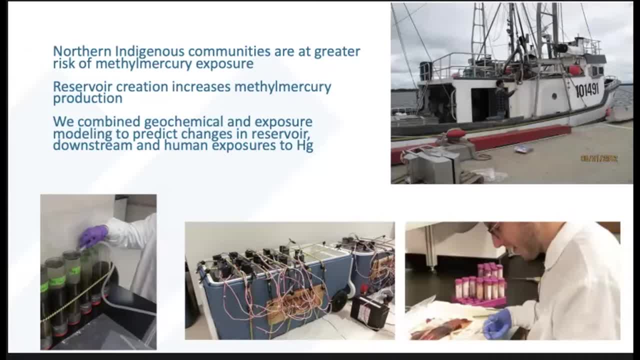 geochemical conditions of methylmercury production in that system, pre-reservoir creation right. So we went out and collected atmospheric measurements, water, sediment, river inputs and looked at how the mercury cycles in that system to understand that baseline level. Then we did incubation experiments. so you're seeing some of those incubation cores here. 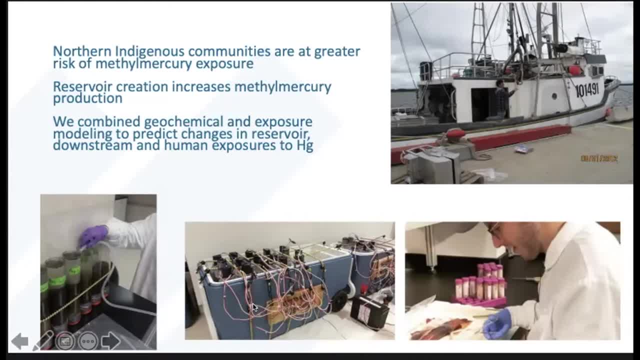 around the area that they plan on flooding. So we took cores and we used the river water that was going to be used to flood that reservoir to estimate, to actually measure by how much methylmercury will increase as the water incubates the soil from that system. We then used 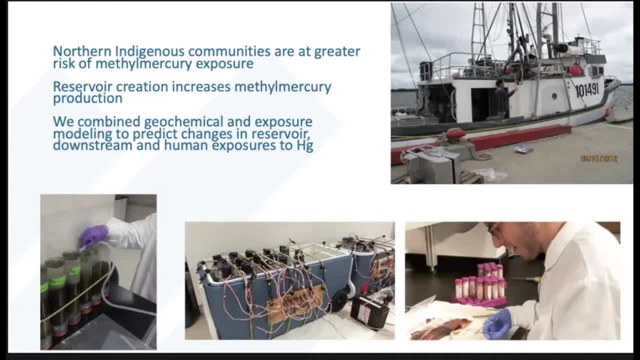 this information to force a model that looks at a pulse of methylmercury following that reservoir creation through that baseline system on which we created a model. And so we combined that with baseline methylmercury exposure level in the community living around the area so we obtain 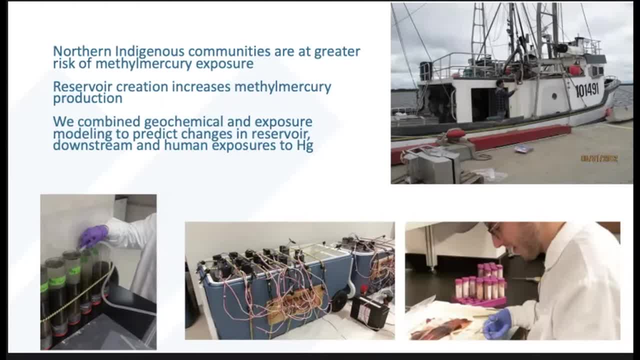 a different baseline level of methylmercury exposure to the area. So we obtained a different baseline level of methylmercury exposure to the area. so we obtained a different baseline information from the community. So they told us how much fish they ate, where the fish was coming. 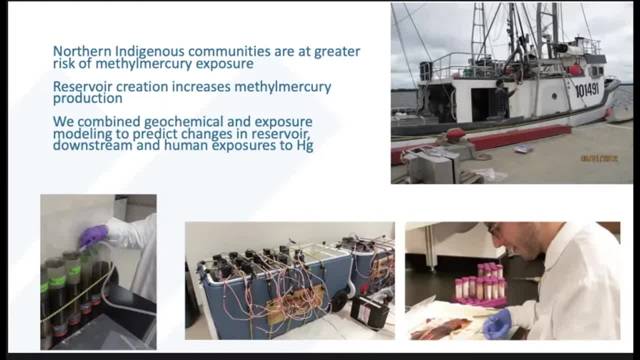 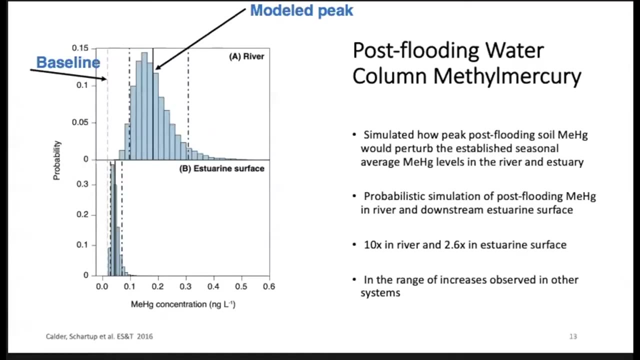 from over a certain period of time. They provided hair samples so we knew what their baseline exposure was and have an idea from which species were they getting most of their mercury- And I'll get to that in a second. And so the next step was: once we had all this baseline information we had. 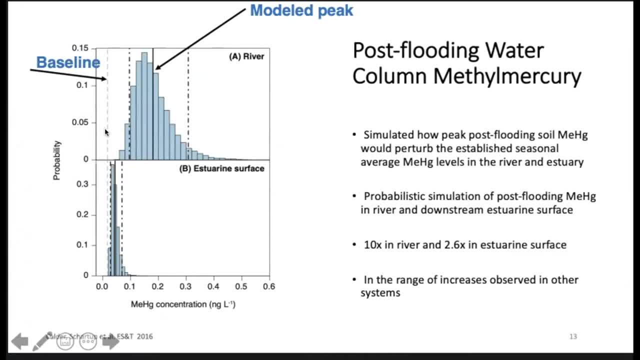 we developed this probabilistic simulation of what will happen if you flood the system and by how much mercury is going to increase in the river downstream of the reservoir as well as the estuarine surface, And we estimated it on average that it will be around 10 times increase in the 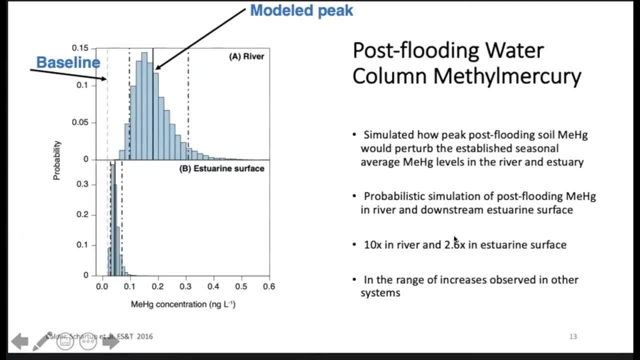 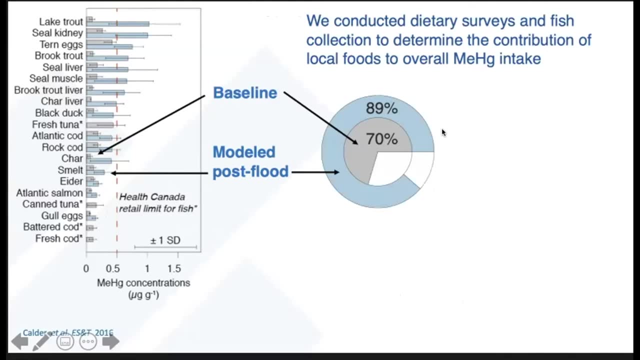 river and about two and a half times increase in the estuarine water. The range here is consistent with what has been observed in other systems. post-reservoir creation, We then propagated it to the animals and the food that people consumed from the system. So 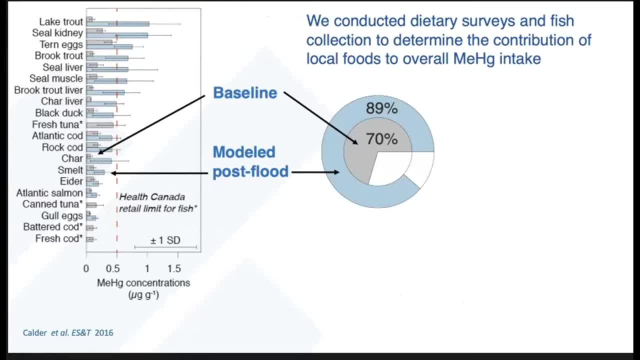 we received a dietary survey so we know what they eat. We also obtained samples from fishermen locally from the different areas of the system so we could measure the quality of the food. And we also estimated the concentration of mercury at baseline. We then estimated based on how much each 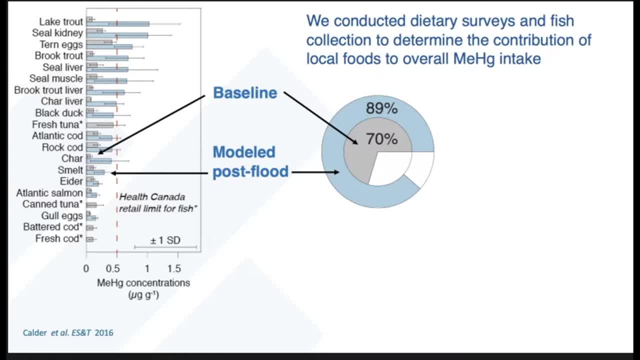 species spends in the different parts of the system, whether it's spending most time in the river or in the estuary or offshore. so no increase there, but a little bit of an increase in the estuary, a huge increase in the river right. We can then calculate how much we expect the 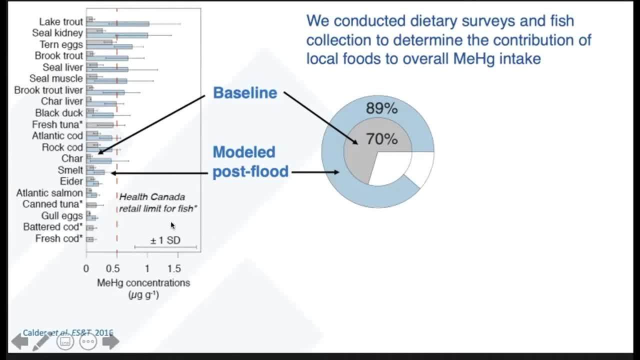 increase to be in the different species that the communities that live around Lake Melville are consuming and expecting, So we can estimate the amount of mercury that you can get from distribution right. The water is flowing and it's going to become a tiny WILLIAMS, so the amount of mercury that you've got is going to be. 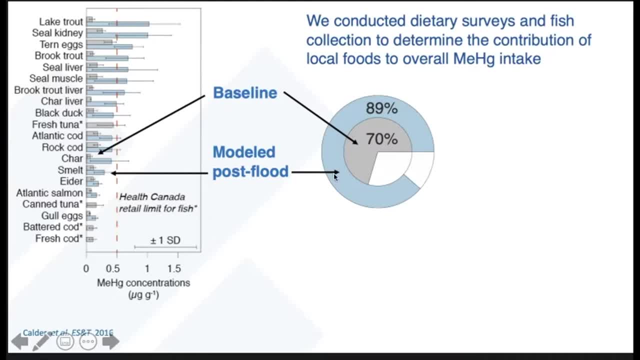 supposed to, And so we had both baseline exposure as well as our post-flooded exposure, assuming that consumption of the different species that people are consuming at baseline will not change in the future. And then the other thing that Ryan actually did. so this is in a somewhat 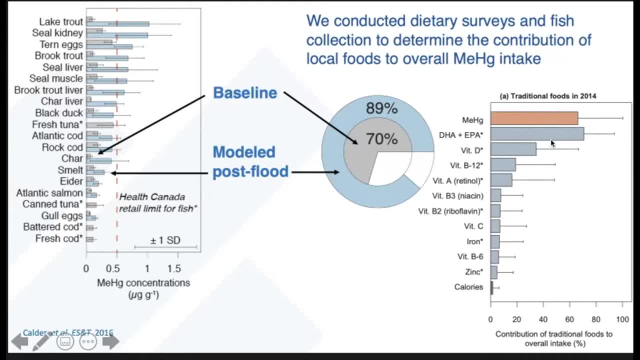 separate study was to look at what is the contribution of traditional foods for methylmercury, as well as all the other things. So we really needed to be careful and work this line where, while we are investigating the impact of the hydro development and looking at how much methylmercury 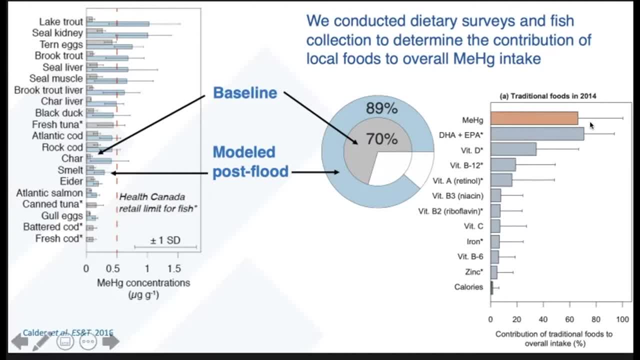 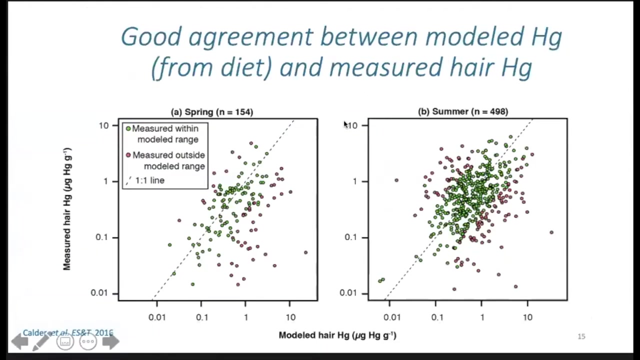 exposure will come from the food is also to really highlight that traditional foods is still a good source of the healthy stuff and that people probably should not replace it with something else that is less healthy than continued to consume traditional foods. So between the measured hair concentration and the model concentration, we found a good 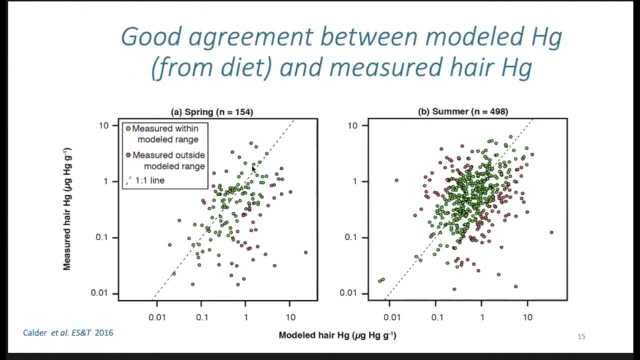 agreement. So we obtained the model hair concentration from the diet that people provided. So they would say, okay, I ate, you know, lake trout and salmon And so on. and then we measure the hair and then we have a good agreement between the two. 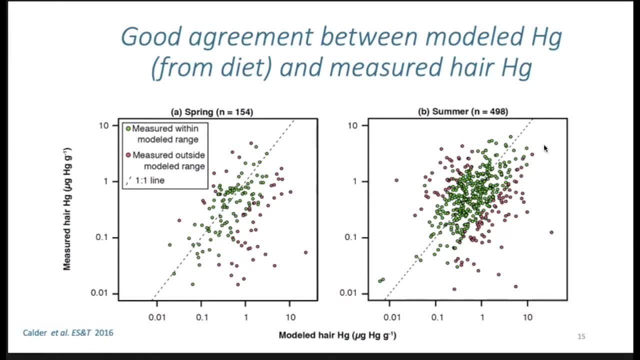 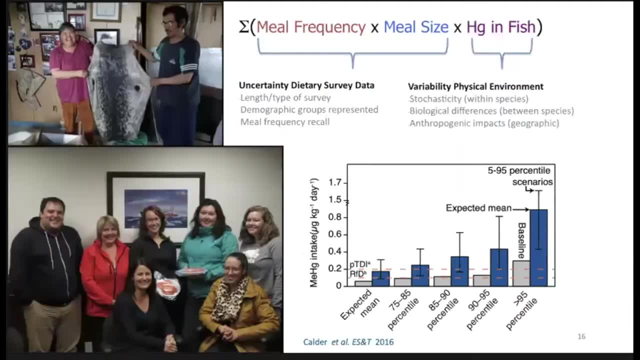 And this allows us to then use the model to predict future exposure, assuming that people continue to consume the same diet post flooding. And what we found here is that, at baseline, quite a bit of the population was already at kind of the limits that are proposed by the EPA in terms of 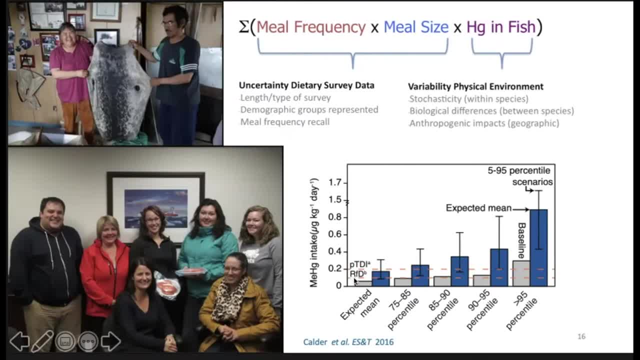 their own needs to make a change. So we have that number of people that are more likely to do this because they're less likely to consume or they're more likely to stop the diet. and this is only when you're measuring those two levels of the population. 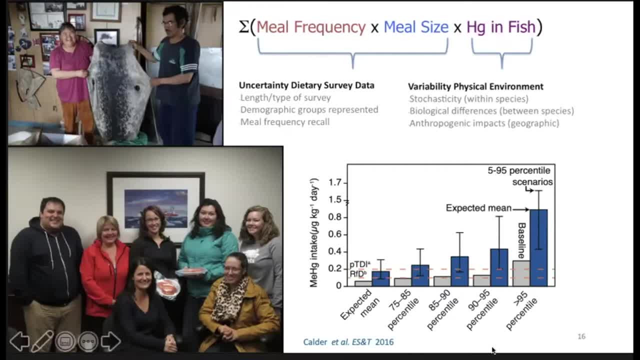 and at the same time, well, that's not necessarily a good thing to do, because you know, we're trying to get as many of those people out of these areas as we can, but we're trying to make sure that they're not. 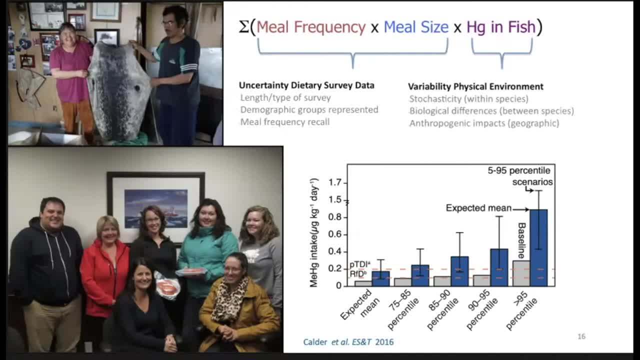 pushing too much of the fish out of these areas. Thank you, more of the traditional foods. versus the younger people had a more varied, less traditional foods, heavy diet, And so they were a little bit less at risk in terms of increased methylmercury. 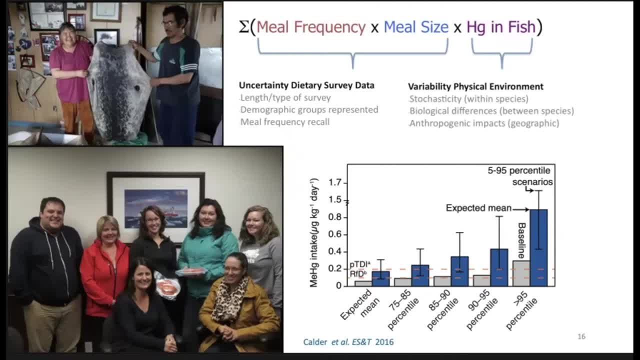 concentrations, And so what? the idea was there is that we need to push for a monitoring of methylmercury levels in the system and thinking about ways to flood and create the reservoir to limit the increase in methylmercury Because, as I've mentioned earlier, the traditional foods are 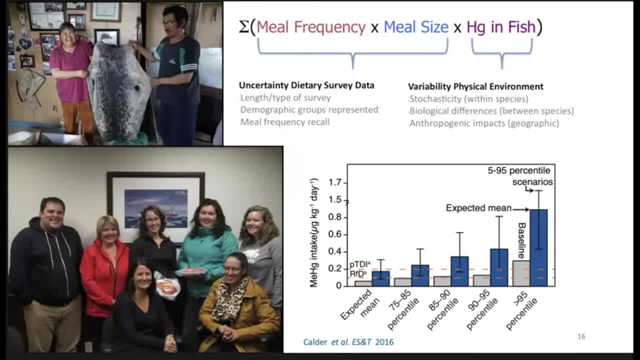 also a source of all these other good nutrients. So the traditional advice of just change your diet is not something that is recommended, both for health reasons, because it, you know, provides vitamin D and so on, but also for cultural reasons, because you don't want people to change. 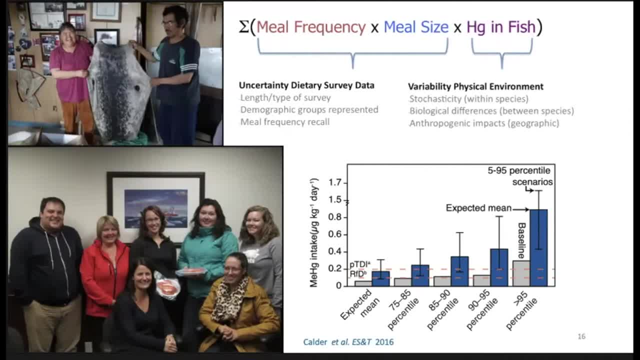 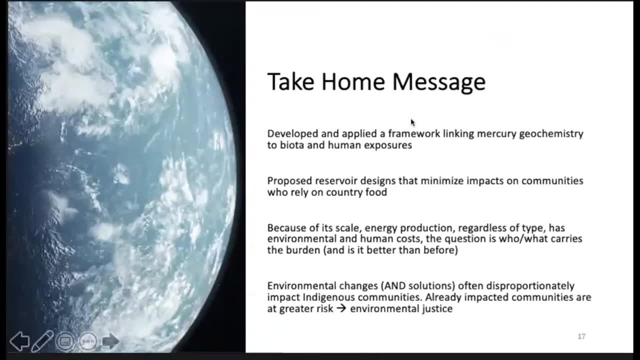 their traditional ways of living just because they decided to dump a bunch of methylmercury in it. pretty much right. So the take home message from this work was that we developed an analytical framework that links the geochemistry to biota, but also to human exposure, and proposed some reservoir designs. 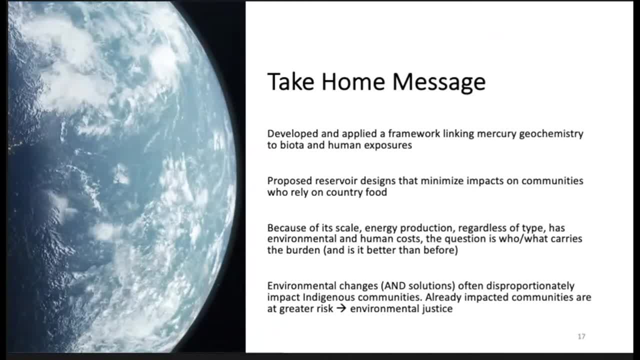 that minimizes impact on communities that rely on country food, such as run of the river, reservoir creation. flood as little as possible. do not flood a lot of land right away, just kind of you know. do not flood a lot of land right away, just kind of you know, do not flood. 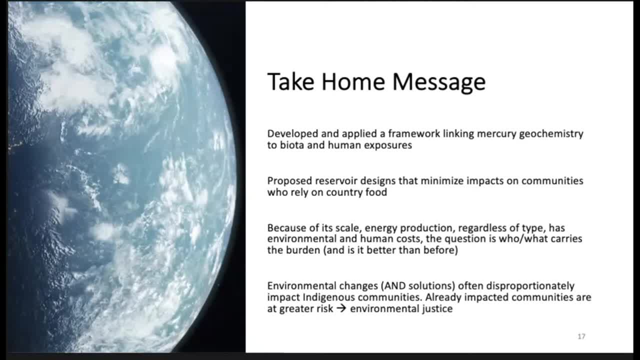 a lot of land right away, just kind of, you know, do not flood a lot of land right away, just kind of like, increase it slowly So you don't have this big pulse of methylmercury that goes into people's waters. And really kind of like a philosophical point here is that because of the 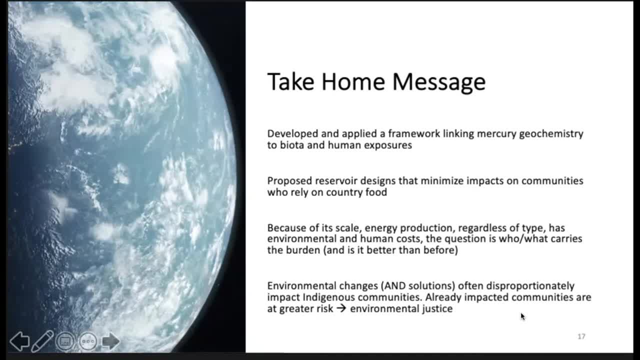 scale that we're looking at. energy production, regardless of the type, has an environmental and human costs. So even though hydro development is considered a green energy source, we really need to think about who is going to carry the burden of those resources. So I think that's a really good. 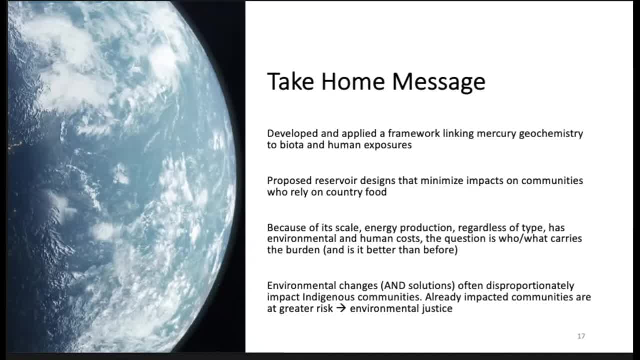 answer, And I think that's a really good answer. And I think that's a really good answer And I think those shifts right. So, while at a global scale, yes, we want more hydro because it's better than burning a bunch of coal that releases mercury too right- I think that it's really important to think. 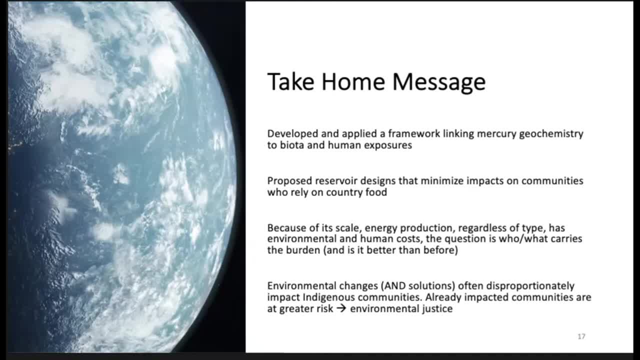 about who are we shifting the burden of those global issues that we're dealing, And very often the burden disproportionately impacts indigenous communities, And so these are communities that are often already at greater risks for environmental change. And so there's, we start going into environmental justice. 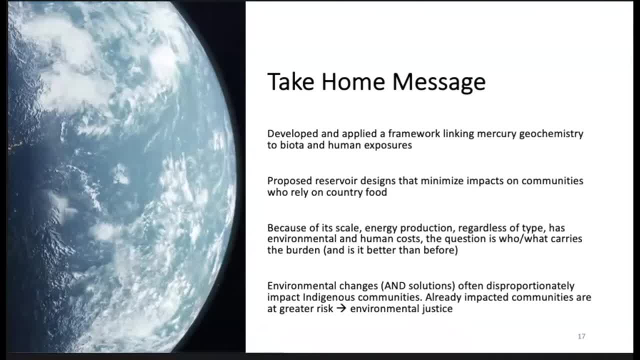 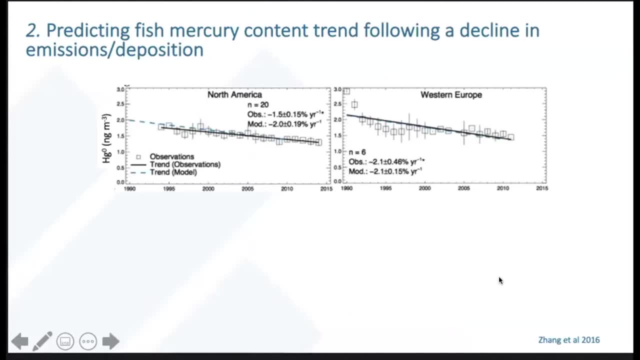 concern here that we really need to be aware of as we're trying to find solutions to climate change. So the second example here is looking at predicting fish mercury content, following the clients that we're seeing in emissions in North America. So this is an example from work from Yang Shu. 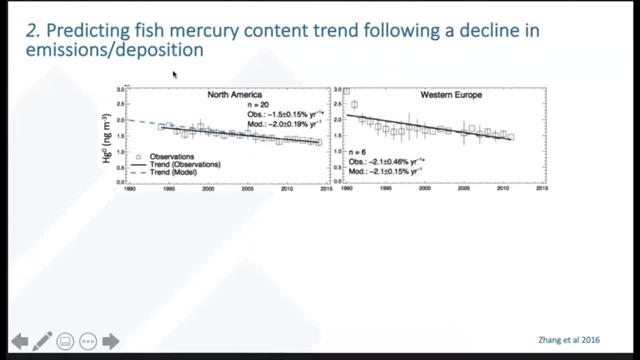 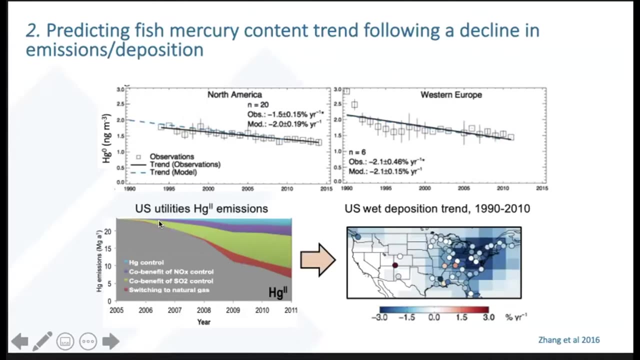 where he modeled declines in elemental mercury in North America, mostly driven by a better control on US utilities of some other contaminants. So we had a lot of co-benefits due to control of NOxs as well as sulfur emissions in the switch to natural gas And this resulted as a kind of like a benefit. 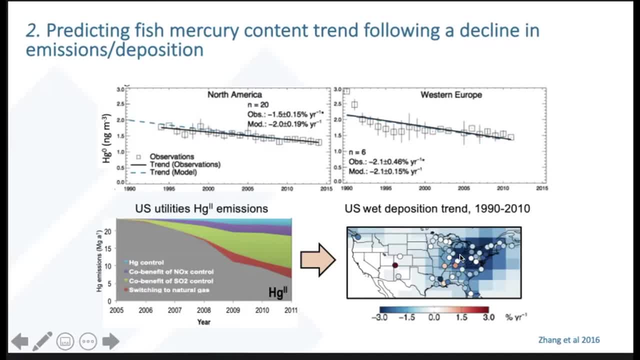 in reducing mercury emissions in the northeast of the United States. So the question was: we're seeing those declines over the past several decades? Are we seeing declines in fish mercury levels? right? Because if we are assuming that we control the mercury emissions, 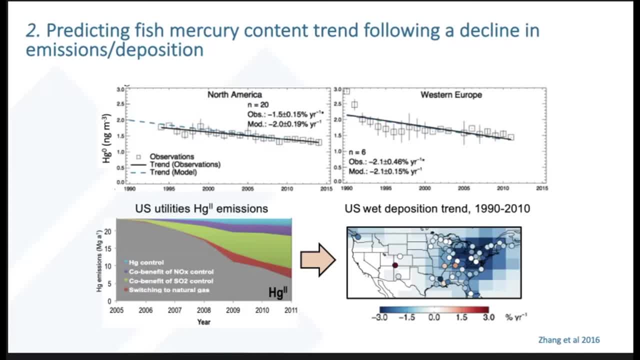 we will have a lot of co-benefits in reducing mercury emissions in the northeast of the United States. So if we are assuming that we will see a decline in fish, then we need to know by how much if that's the case- And one of the things that I was concerned about is there's all these other 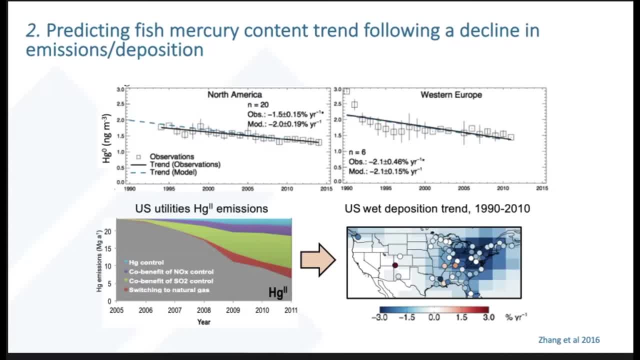 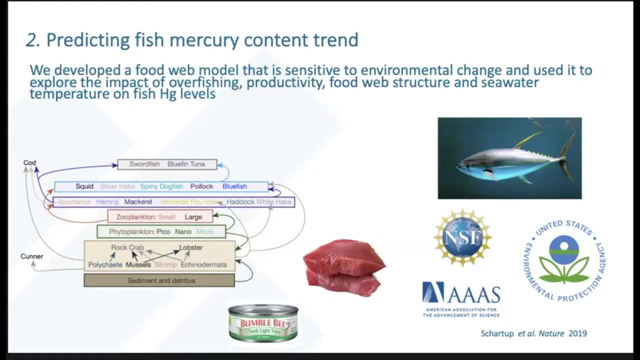 environmental changes that are happening in this region at the same time, such as seawater temperature, increasing changes in productivity, inputs of organic matter into the northeast Atlantic Ocean. So the question was: how does mercury levels in the fish change, knowing that we have all these other changes at the same time? So in order to address some of that, we developed 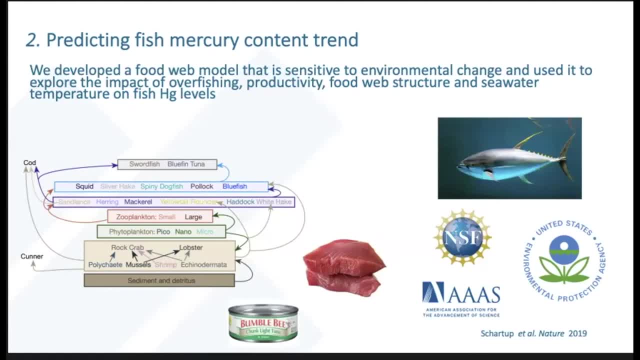 a food web model that is sensitive to these environmental changes and used it to explore the impact of overfishing, increased productivity or changes in productivity, food web structures, seawater temperature, et cetera, on fish mercury levels. So the model is based in the Gulf of Maine. 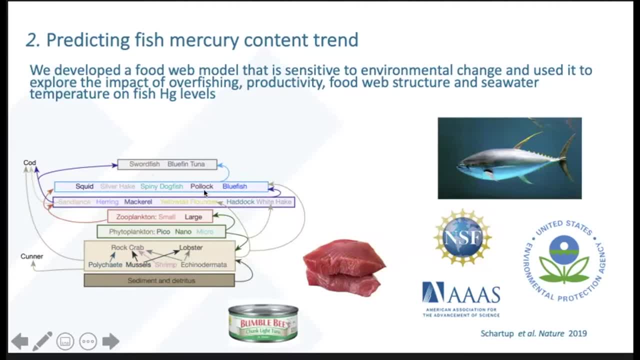 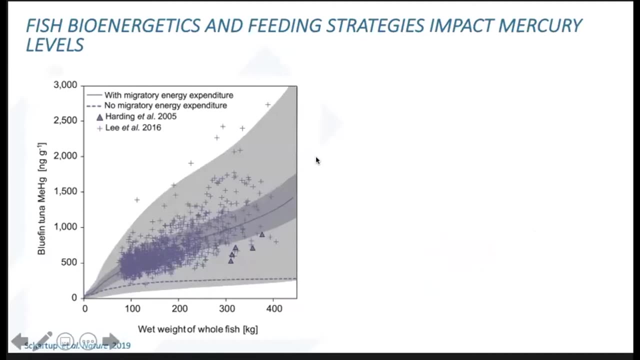 And the reason for that was because we have a lot of data that NOAA has been collecting on fish stomach content- just changes in the food web structure- And then we had enough mercury in fish data to evaluate the model And so kind of like the top of our trophic level in the system was Atlantic. 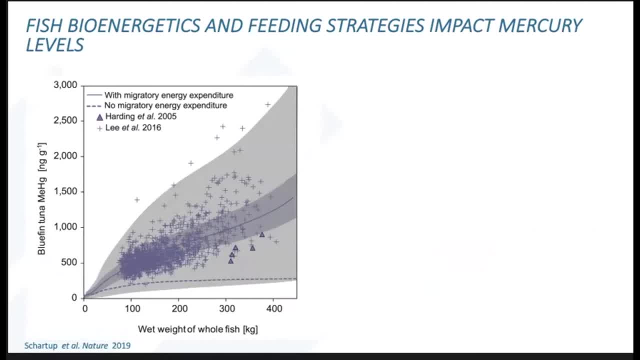 bluefin tuna, And then we also had swordfish and a few other large predatory ones at the top And, as you can see here, had a pretty good amount of mercury, And then we had a lot of mercury in the sea as well, And so each of these different data points the fact that we have an infinite amount of 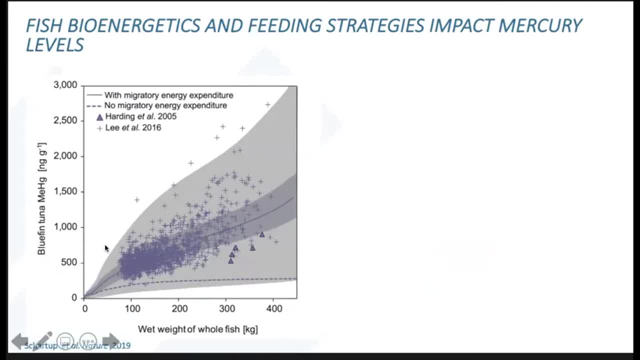 data, each data point. here is a bluefin tuna And we kind of worked with trying to understand, like: what are the drivers of these changes of mercury levels in the fish? Is it concentration in seawater? Is it the organic carbon content? Is it? 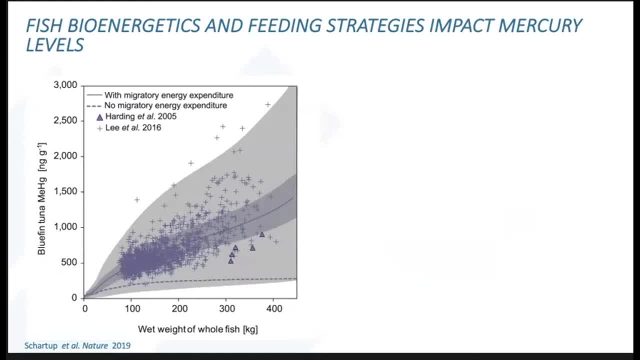 the biologetic of the fish or the structure of the diet- What are the different fish you're eating- And we have some data that we've been working with, like we have a unique starting point. a lot of We worked through that for different species and we did a pretty good job at modeling all the fish that we had in the food web model. 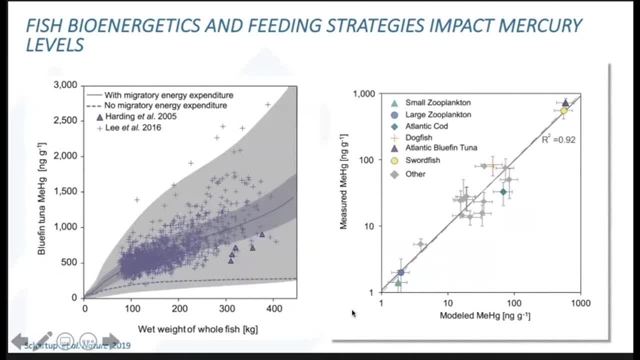 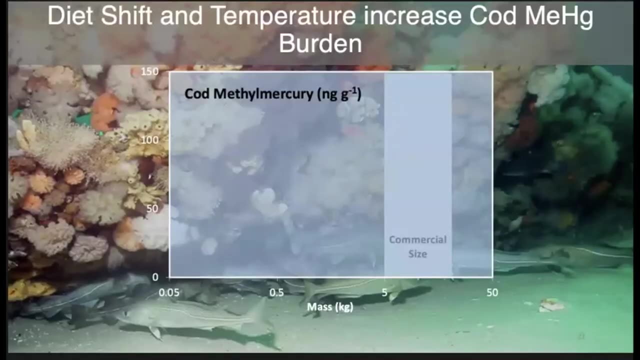 And so the idea there was that now that we have a functioning food web model and we know how the fish kind of acquired a murky by eating each other under the different conditions that we can change in the model, we can then try to see what are the possible changes over time and how do they impact the murky level in the fish. 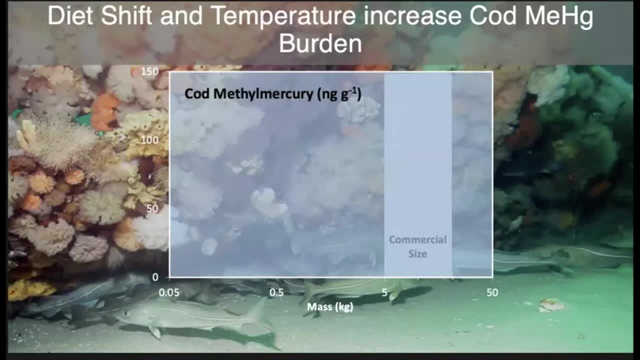 And in a way we were hoping that it would explain why fish species that live in the same ecosystem, So in theory, seeing the same declines or increases of murky levels, how come they respond differently? sometimes Some of them see an increase in murky levels versus others seeing a decline, even though they live in the same ecosystem, that is, overall seeing a decline in that position. 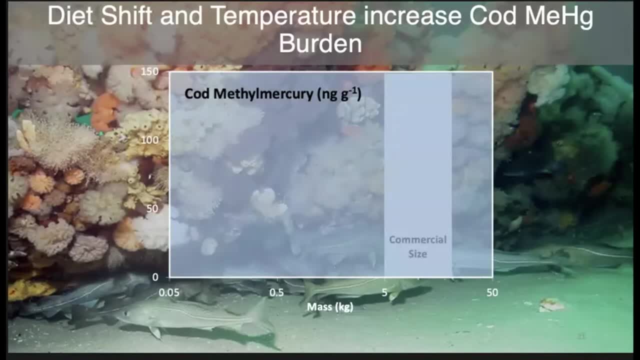 So this is some of the things that we were running into that we're trying to explain with the model, And so an example here is cod murky level over time. What happens if you increase the model seawater temperature by one degree, you see that cod murky levels increase just as the temperature of seawater changes. 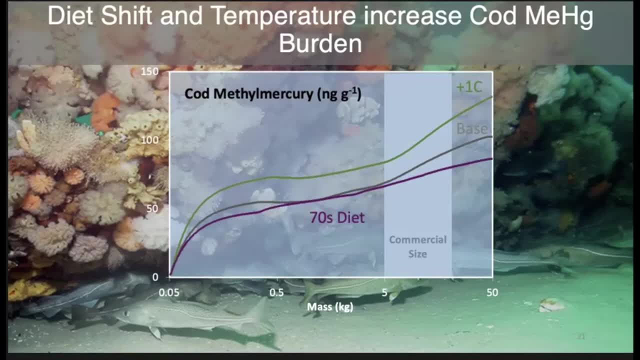 However, if we switch the diet from cod for what we had at base, which was the 2000 diet, to a 70s diet, you see that the 70s diet actually had a lower methylmercury in cod than the 2000 diet. 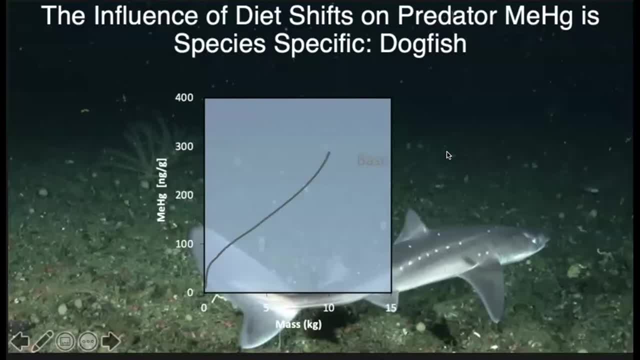 However, when we did the same thing for dogfish, we saw the opposite trend where, from the 70s to the 2000, we see a decline in murky level. This is fish that are living in the same ecosystem, exposed to the same waters, the same murky levels in the water, but they're seeing that decline. 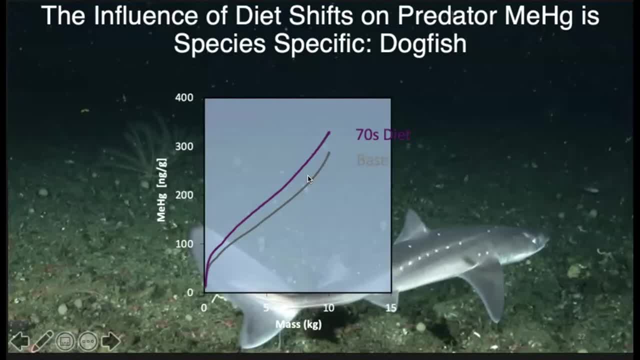 And that's just driven by the fact that, as the herring, because you remove certain species from the ecosystem, so in this case it was herring- those two species that used to rely on the murky level to survive. they're now living in murky levels. 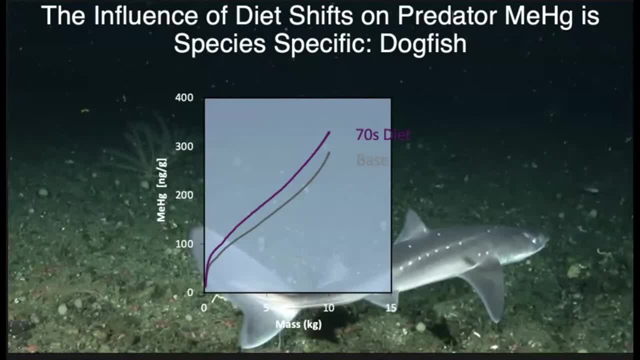 on eating herring, switch to a different prey and so, depending on the prey that they pick, their mercury levels go in different directions. so that's. we thought that was really interesting, but overall the temperature increase on all the species that we look like tend to increase the methylmercury levels. We did something similar for Atlantic bluefin tuna, except. 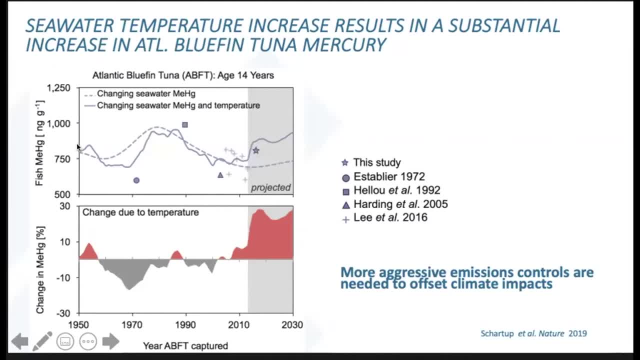 that in this case we had kind of like an historic. we forced the model with historic seawater temperatures as well as methylmercury concentrations and look at how the combination of both changing seawater concentrations of mercury as well as the temperature impact the bluefin tuna methylmercury levels. What we found was there were ups and downs driven by 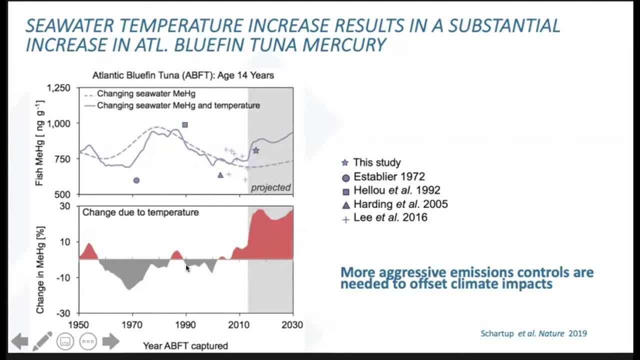 both the concentration of mercury as well as changing temperature. but one thing that was interesting is that when we projected into the future and kept the methylmercury and seawater almost close, the temperature would increase and the temperature would decrease, So we were able to. 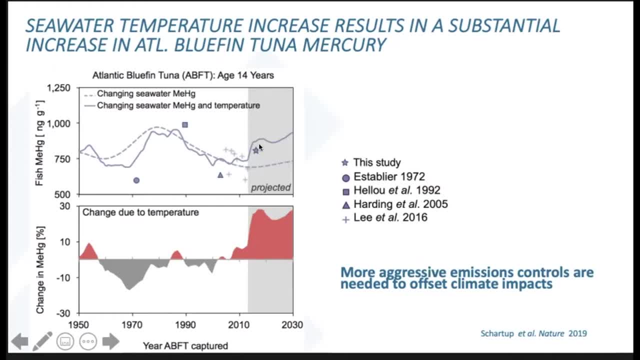 see a constant, so that dotted line. here we see an increase in methylmercury in bluefin tuna, just driven by warmer temperatures, And so the warmer temperatures are impacting the bioenergetics of the fish and really the bioenergetics of in the entire food web, as you can see this fish below it see. 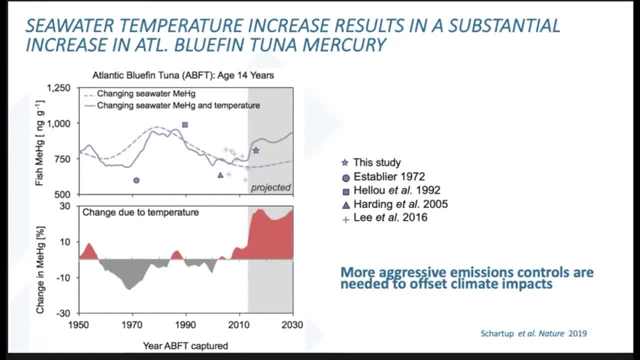 their increase in methylmercury due to increased seawater temperature. and sitting on the top, the bluefin tuna kind of integrates that whole signal from the bottom of the food web, And so what this is telling us is that when we look at the temperature of the bluefin tuna, we see that 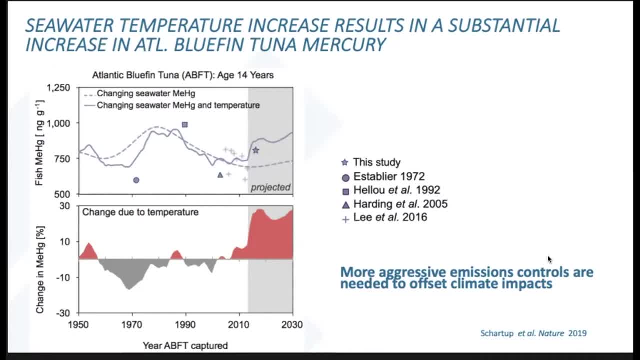 we want this. we want to see more aggressive emissions control. that we can't assume that if we reduce emissions by 10%, we'll see a 10% decline in methylmercury level in the fish. What we're going to see is that these other environmental changes may either enhance or 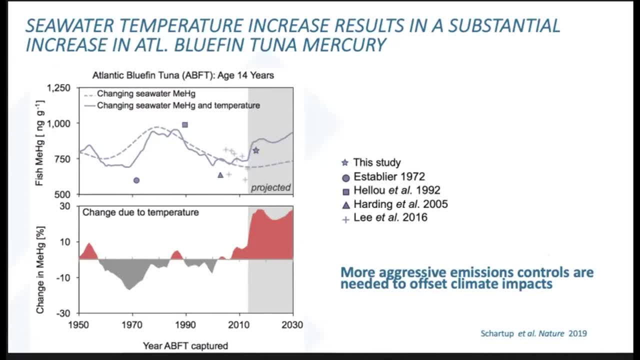 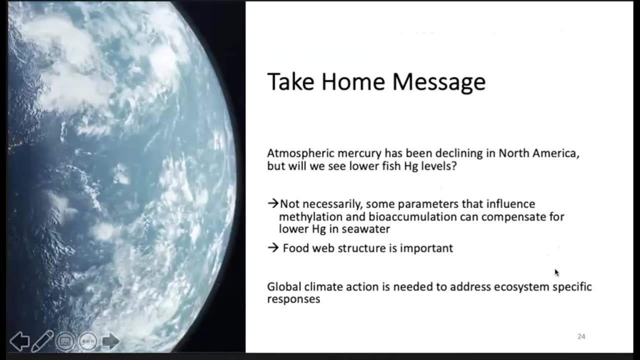 offset some of those changes in methylmercury concentration. So we really need to understand those other environmental parameters in order to effectively reduce methylmercury level in seafood. So the take-home message here is again that despite declining mercury emissions in the North America, we don't know whether we're going to see lower fish levels, because we don't really. 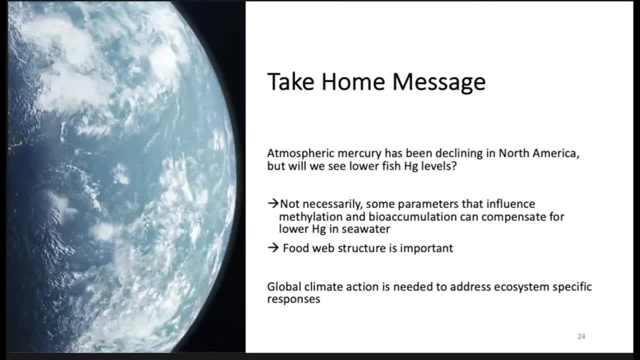 have a good grasp how these kind of ancillary parameters are driving changes in uptake and so on of methylmercury and the food web structure itself is important to be able to quantify that. One thing we know for sure is that global climate action is needed to address some of 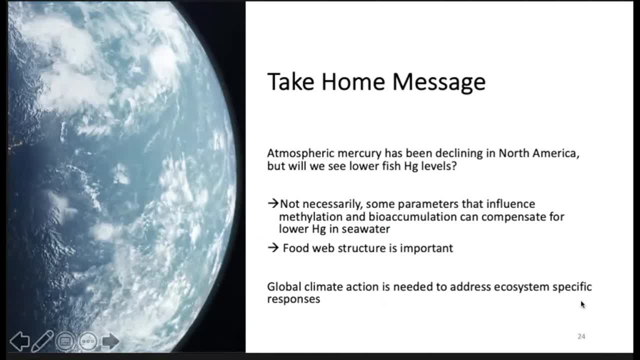 these even ecosystem specific responses, because the increase in temperature in the Gulf of Maine is a global climate action issue, that the temperatures are rising and so we need to have a control on that. The other thing is that those two are related. right, the temperature rising because, in part, we are burning fossil fuel, the same fossil fuel that is emitting. 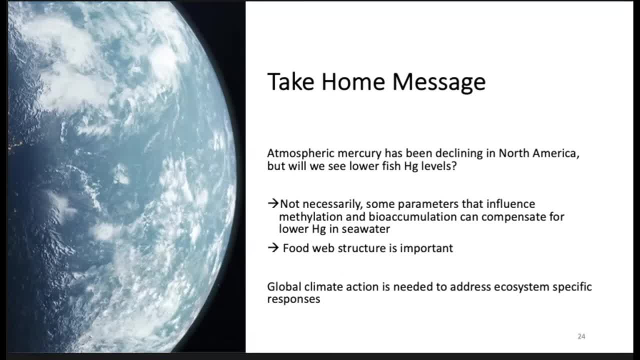 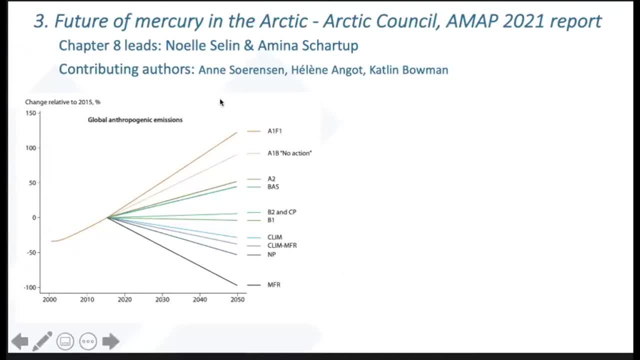 mercury into the environment. so if we have those under control, the mercury emissions will also decline. And this is kind of my segue into my final example- is: well, what is the future of mercury in the Arctic following changes in those emissions into the environment? and so what we did here? so 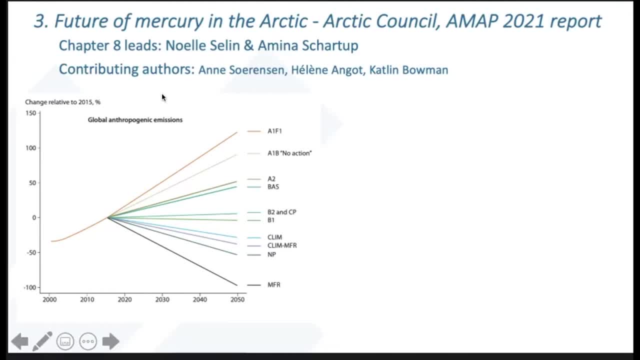 the leads for this chapter, Noel Slim and myself, and then we have contributing authors, and so we use several anthropogenic emission models. in this particular case, we use these three, which was the a1b1, which is no action, assuming we're not doing anything to reduce mercury. 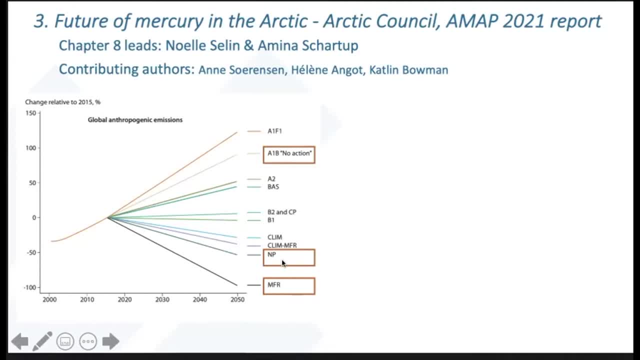 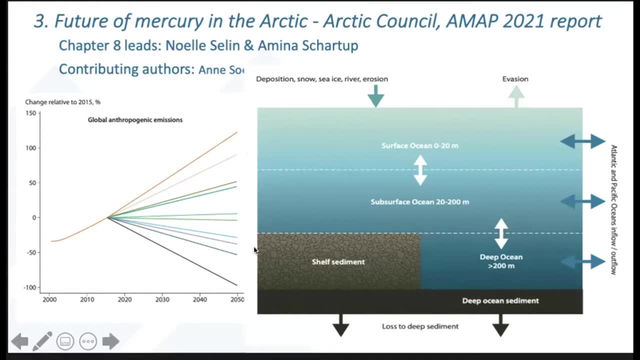 emissions. we and we have two control scenarios and then we use the deposition from this emission scenarios to drive a model, relatively simple model box model for the Arctic. it was based on Anne Sorenson's 2016 GBC paper, So I am going to show you how we have. 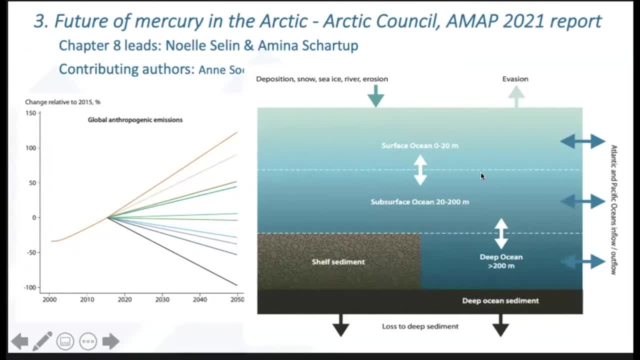 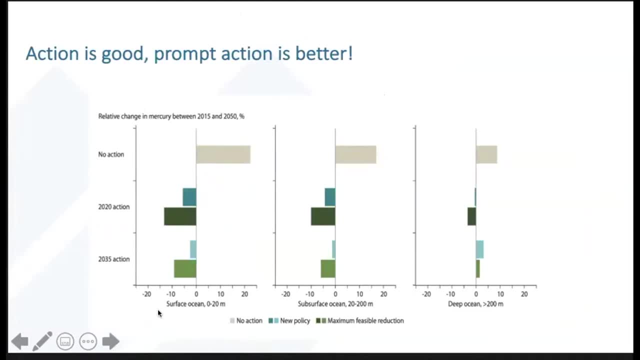 This picture here In our second slide. So I will start with this side so that this is the deep bottom. you all can see the unusual piece. And this is the deep bottom. you can see that it actually was protected from extreme warming And this is our thermal surface of age temperature. As you see it, on the front left And these are some of the third types of massive ice layers and reactions are we can actually see. I'm going to walk you through these three. so this is the surface, this is kind of mid depth and this 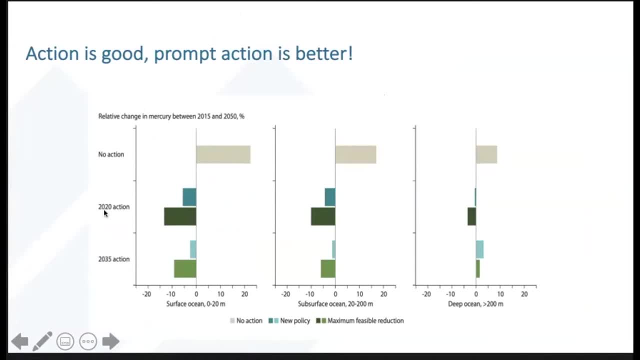 on this side, it's a decrease, and these action means: what if we act in 2020? or what if we act in 2035? it was 2020 because at the time it was 2019. we're working on that, so we're already behind. 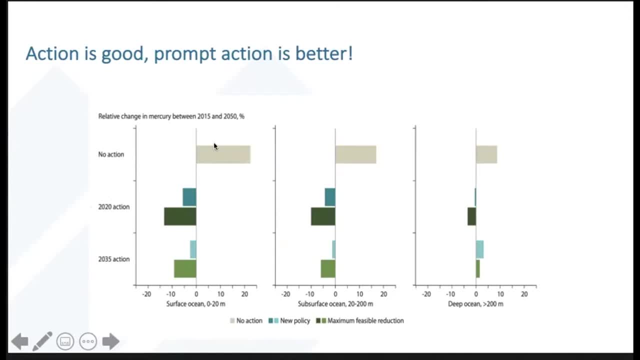 the times, it's just crazy, and so what this is showing is that, in all cases, we will see an increase in mercury in the arctic ocean, whether it's in the surface of the ocean, if we don't do anything. however, if we do act, we will see an overall decline, even if our action is relatively. 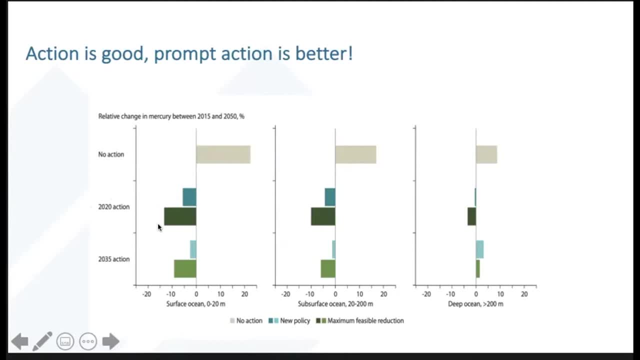 modest, although the sooner we act, the more of a difference we can make, and that's driven by the fact that mercury builds up, which was told you earlier. it's a legacy thing, so the stuff that we're releasing today is adding on tomorrow. so the longer we wait, the more we will build up in. 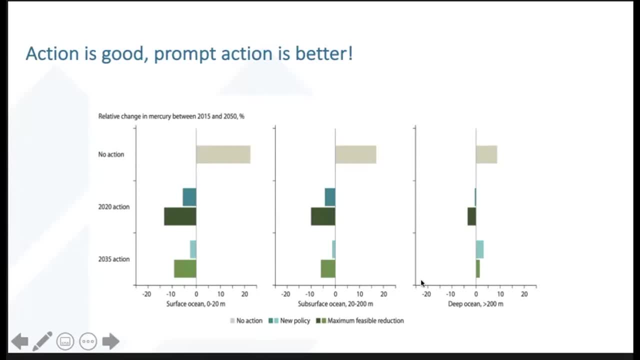 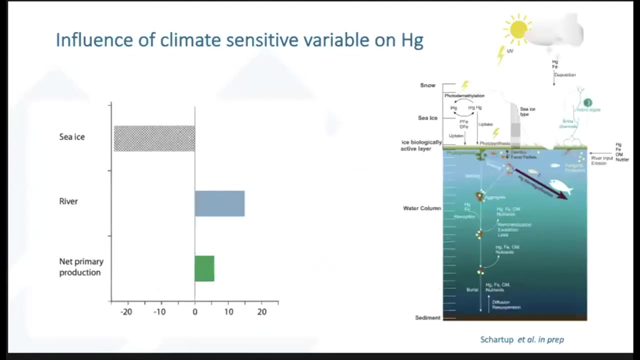 the system, and so there's also a lack of time as we go with depth, because, as you can see here, you know 2020 for the deep ocean, there's not much of a difference. that's because, well, it takes a while to impact the deep ocean and, of course, i was curious to see what is the influence of the 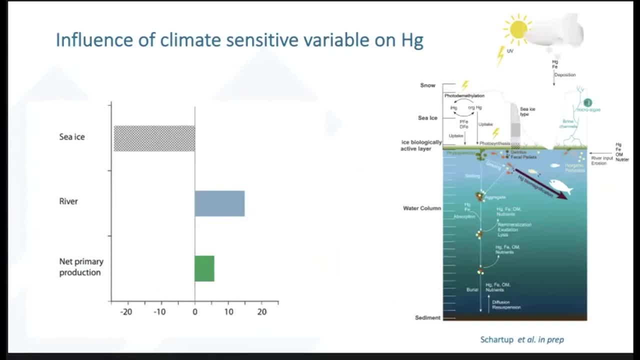 climate sensitive variables on mercury, and we know that in the arctic sea ice is changing, river input is increasing and primary production has been increasing too, and so we wanted to see how are these other changes going to impact mercury level? we know that sea ice is kind of serving as a cap on the air-sea exchange, so maybe removing sea ice we'll see. 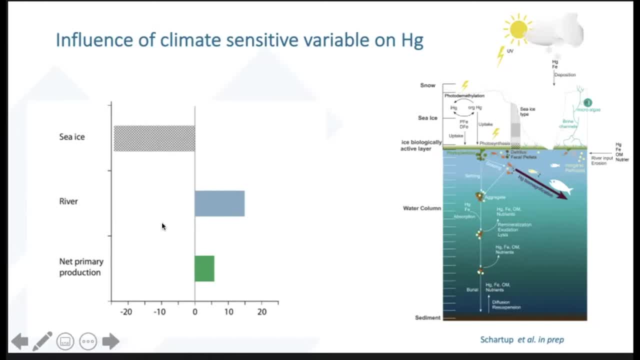 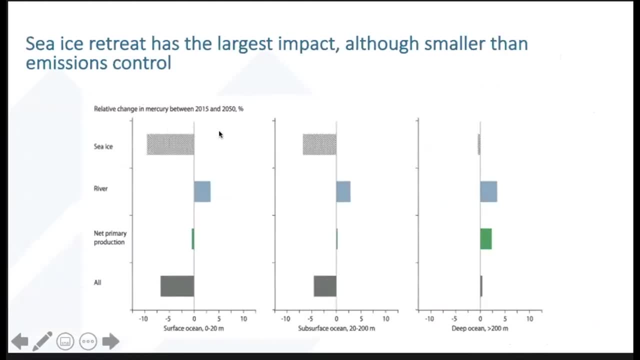 more evasion of mercury, i don't know. so that was the idea, kind of playing around with those environmental parameters and see what we see. and what we're seeing is kind of it's a similar plot, so this time, like you said, surface, mid and deep ocean, but this time we're looking at the impact of 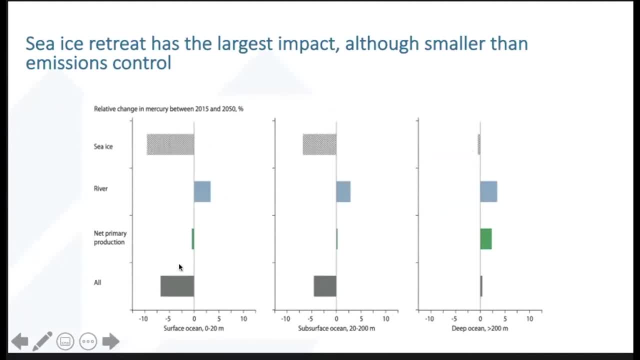 sea, ice, river and net primary production is also all over the top. maybe it can really be fixed as about four hundred meters later. so i feel like we're going to want to increase this amount, but i think it's Firminaking, I think it's going to become much more multiś and be a ride gonna. 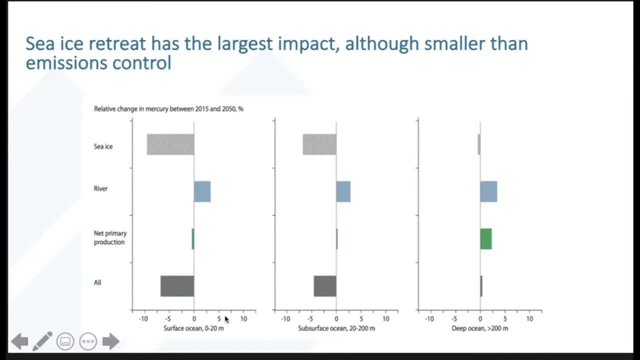 pass it into theめてqual area also make sense, but you have seen a reduction in current sea icetro bride l, but I think that this is going to therefore being a catch-up from filthy activity which turned to double them together. as you can see here, the scale is smaller than what we had with the emissions, so 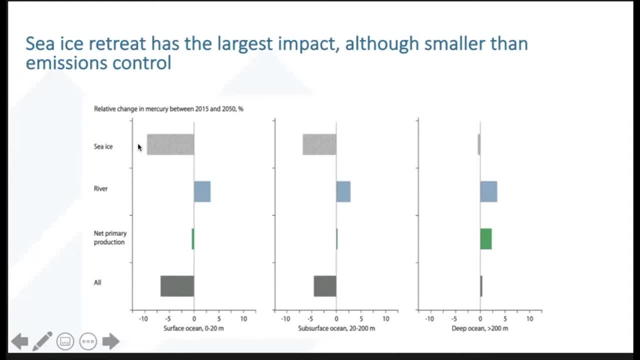 what it's really saying is that, um, those environmental parameters have an impact on the mercury levels in the arctic ocean, but it's smaller than the emissions control. so we still again go back to: we want to control emissions of mercury into the environment, so um the cis. 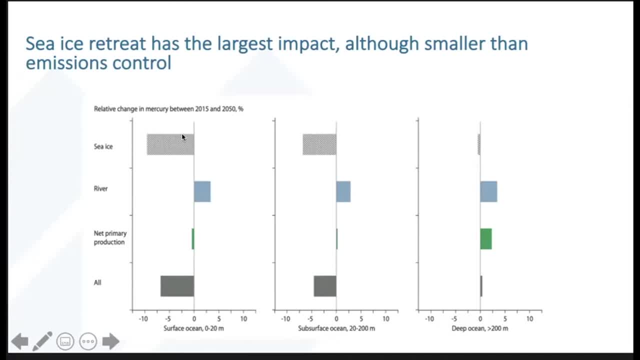 really has the largest impact here on the mercury level and the impact is in the correct direction, which is a reduction in the mercury levels um in the arctic ocean. you will know that sea ice and primary production are related. when we're doing this work, we did just did not have the the model. 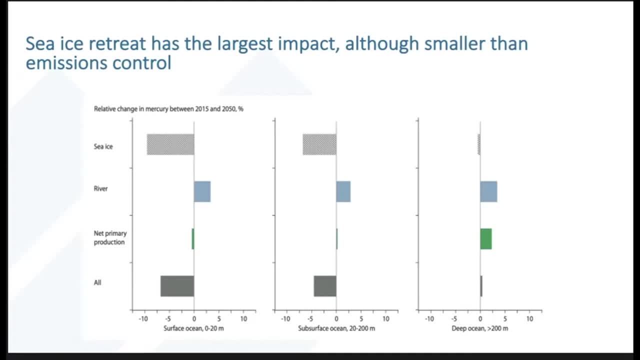 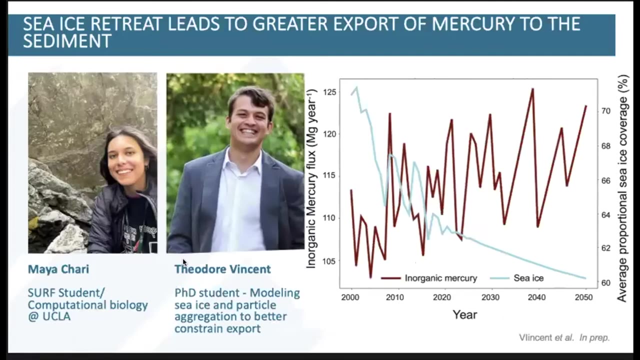 in place to have them coupled. so we are we're looking at it independently, but we know that as the cis is changing, that it also impacting the net primary production. so this is actually something that my students are working on right now- is developing like coupled framework that actually will combine. 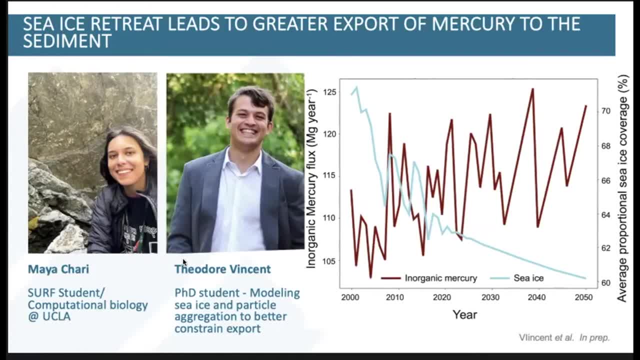 all these different changes and also looking at what this means for methylmercury production. so we had a summer intern, maya, who's a computational biologist at ucla this summer working with my phd student, theodore vincent, and who is modeling sea ice and particle aggregation. 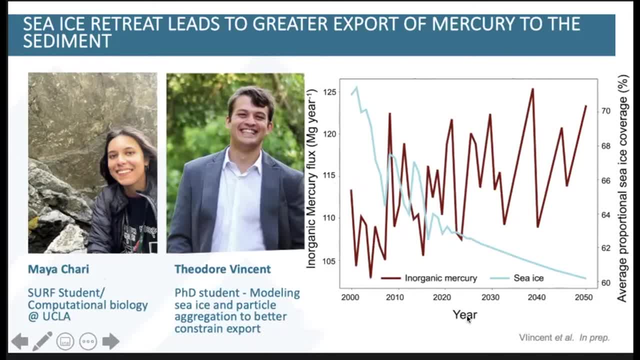 to really help us better understand what's happening, and that's some of their preliminary work where they're looking at uh to changes in sea ice over time and how it impacts inorganic mercury export in the arctic ocean. as you can see, we are seeing more export and removal of mercury from the 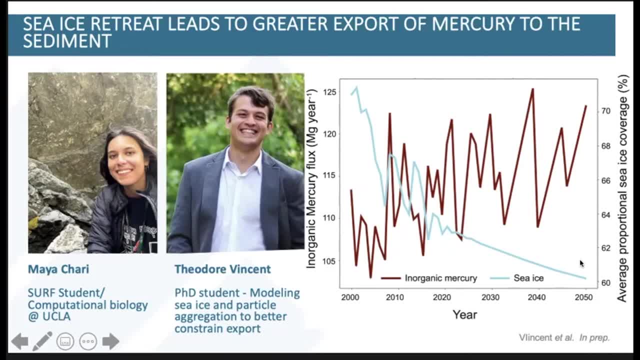 surface ocean as we see that decline in cis and i guess it's kind of a positive spin on this. i don't know, but on this i will say thank you for your attention and i will take some questions. perfect, yeah, thanks, amina, that was great. um, i guess. 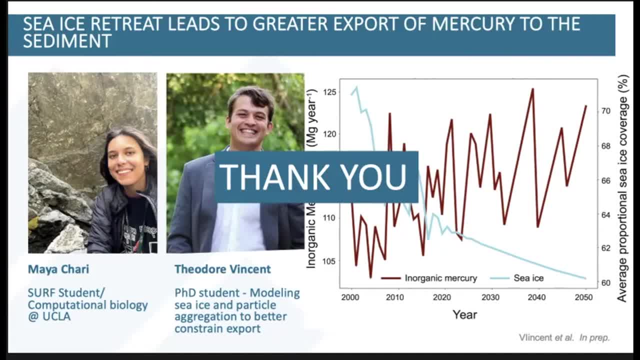 maybe going back to your work in labrador, one of the things you touched on was how difficult it is kind of to do mercury research in the context of food supply security in more remote communities. do you have any kind of tips or things that you use on how to actually 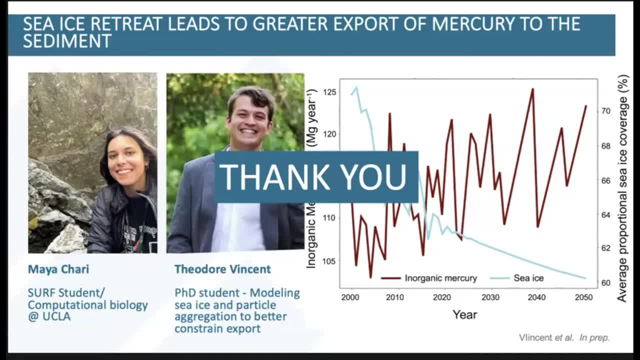 communicate those results to the communities in terms of balancing the risk versus making sure that people continue to eat their traditional foods, yeah, uh. so one thing that i'm really looking at that, uh, i did not know at the time, i know better now is, but we kind of did that. well, what i do, 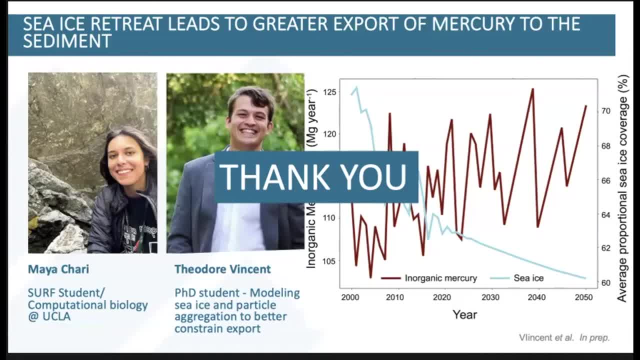 did do is having somebody who is on the ground, who lives with the community, and just explain what our founding and have somebody who is connected with the community to actually transfer the information in a balanced way through how they understand what we are saying. i think it's really so. the our issue was, and still is, is that. 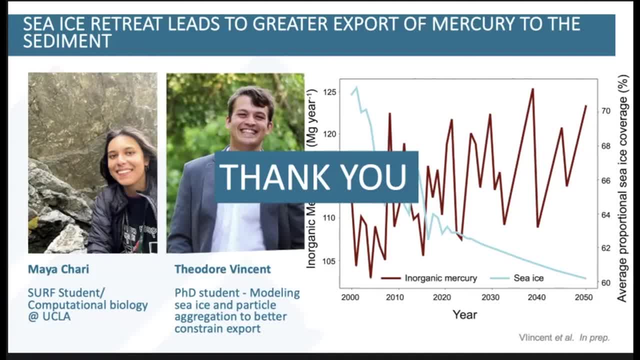 overall. um, i think the traditional foods are are better than alternatives that you know. if people could switch to you know whatever, you know healthy alternatives, uh, then that would be okay, but that's not happening for many socioeconomic reasons. right, really expensive to have access to you know fresh vegetables. sometimes they're not even there, uh so, uh, having you know food from the land. 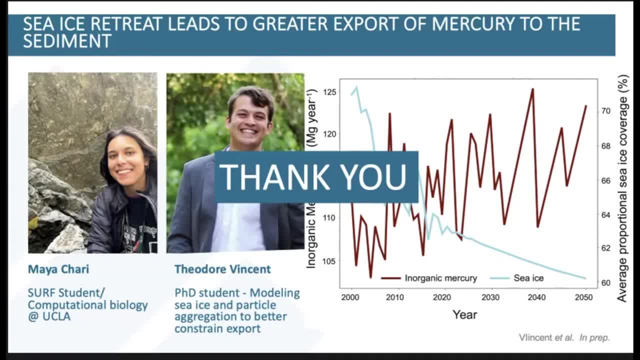 still the best option. so i don't think that we could uh, we can just tell people don't eat it, which is some. what if some of the people would try to suggest uh, at the like, um government level, where they're like, oh just you shoot food advisories and people stop eating. it's like 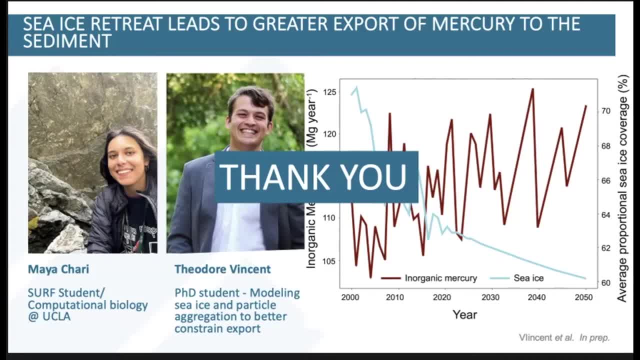 okay, but what are you gonna eat instead? right, you can't do that. so i think it's just being very clear from the get-go- is: continue to eat this. this is not the. the effort shouldn't be on on what people should or should not eat. the effort should be: can we make sure we? 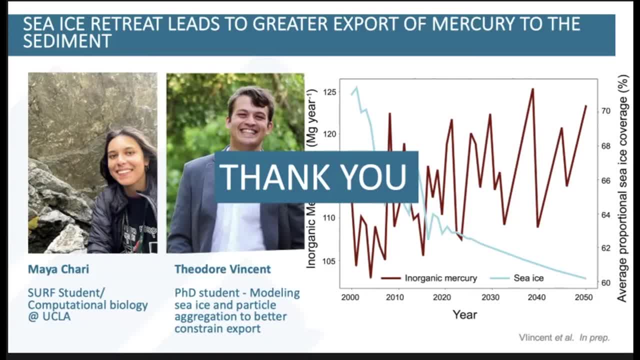 don't increase the mercury level, like that's what we want to see. can the industry or whoever is doing something, they're not, do what they're doing or modify what they're doing so we can make sure that the mercury levels does not increase in the system, and that's clear? 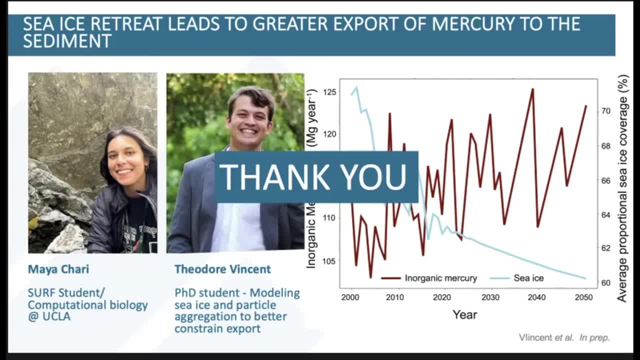 i think we have a follow-up question from colette vapnitz. hi, amina, yeah, um, thank you very much for a super interesting talk and a very clear presentation. um, i had to follow up to kira's question because it's something that i grapple with a lot, working with communities and 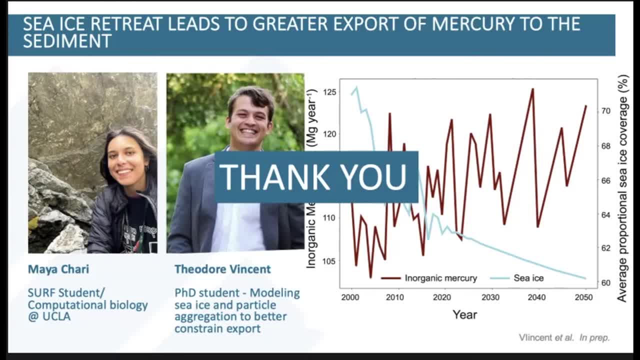 finding these sort of um as a scientist really interesting things um or results in terms of, you know, concentrations of um, of pollutants in in fish, but then also realizing the importance um that these fish and invertebrates and other animals have in people's diets and livelihoods. i 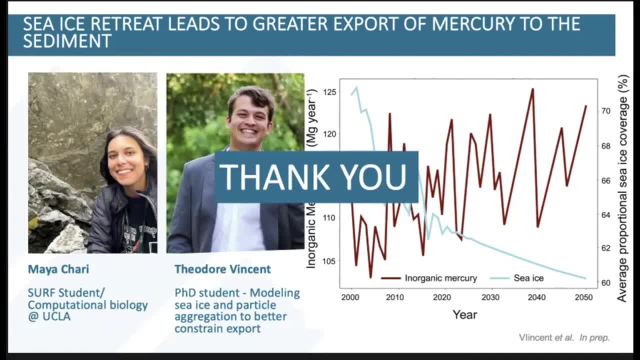 think it's really important to think about how these fish and invertebrates and livelihoods can be used to improve the health and well-being of these fish and other animals as well, and so i was wondering whether you're engaging at any point as a scientist or as a communicator. 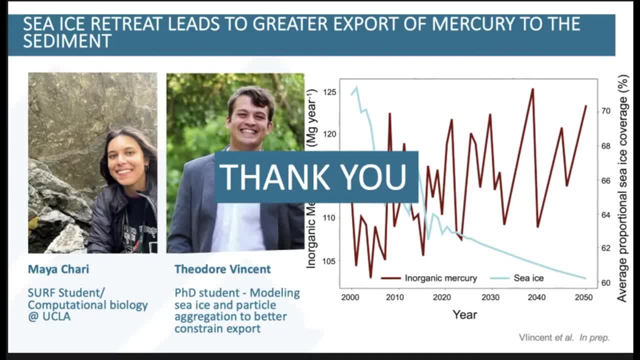 with some of these communities pointing out exactly what you say, because i think a lot of the time the message is very clear like: oh you have, you have methylmercury. it's dangerous, don't eat it. but actually in a lot of cases not eating it is way, way worse because of the edha and epa. 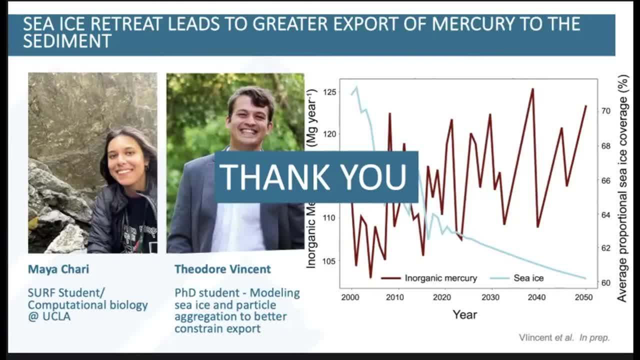 fatty acids, composition of these fish, um to their health. so do you engage at all with some of the c dimensions of this and and mitigating some of these sort of drastic reactions, or are you more taking a sort of step back from that? yeah, uh, no, i'm not engaging in that um and in a way it's i. i. 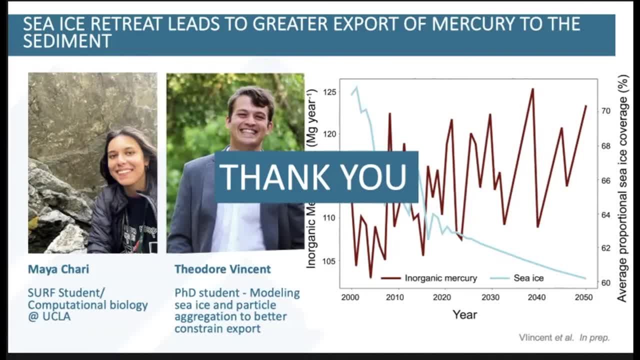 it's not, it's not by choice. i think it's mostly through the circumstances of you know the academic academic requirements, right. so, um, it's something that i definitely want to engage more so. actually, i've had some colleagues where we sat down and thinking about how can we write this down, how can we, you know, can we transfer? 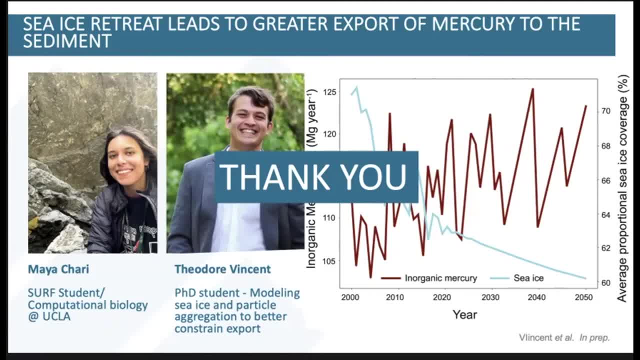 this information right and i've i've. one of the reason i went to nsf after my post-doc was that i wanted to connect with the federal government, people who were engaged in this type of conversations, who were engaged with the communities and, and i think, learning about how exactly do you. 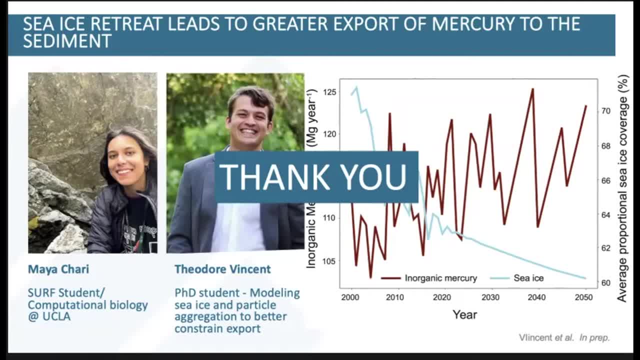 uh, pass along that kind of information without making a mess right. so that's something that i'm really concerned about, and so, in a way, i stayed out of it out of um fear that i don't, i'm not equipped enough to say the right things the right way, and so, um, 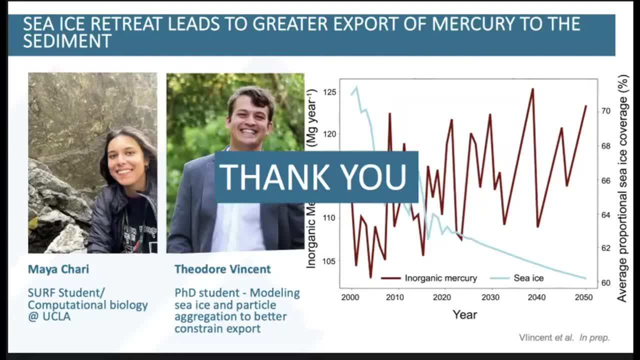 i want to do this now. the question is how to do to, to learn to do it well. um and- and this is something that i'm actually really interested in on a scientific aspect- is: how do we, as geoscientists, learn to walk this line like, not get excited by our results? 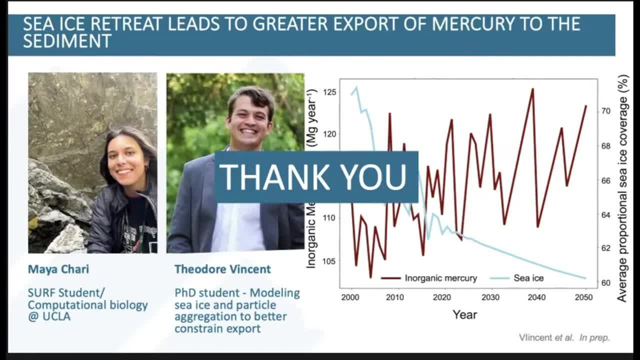 and and be able to kind of like broaden our own understanding of how our results fit in people's lives. and sometimes we're like so narrowly focused that we kind of lose the big picture, um and forget that there are other things that people have to balance. so long answer to your question is no, because i 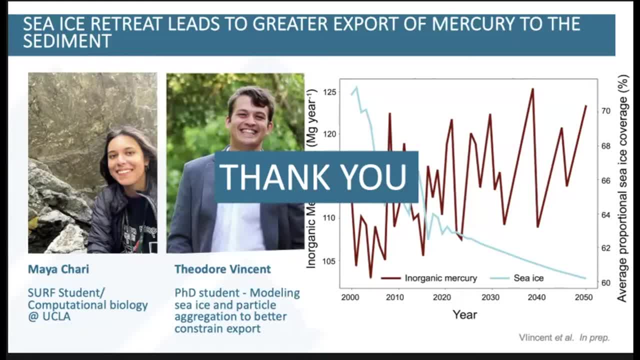 haven't yet figured out how to communicate this well, thank you, i think the next question is from andrea fromel. can you ask the question, andrea? yeah, thanks so much for great presentation. i mean, i really enjoyed it. i had a question: you had uh temperature in your models. 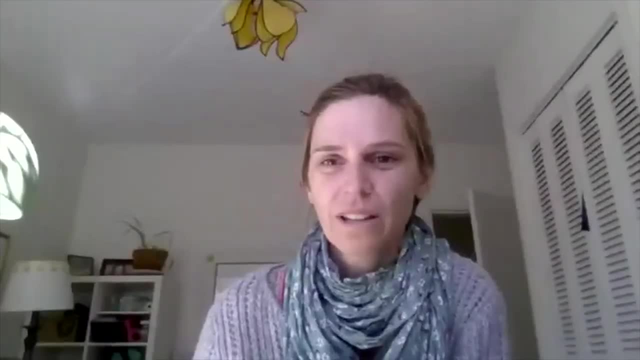 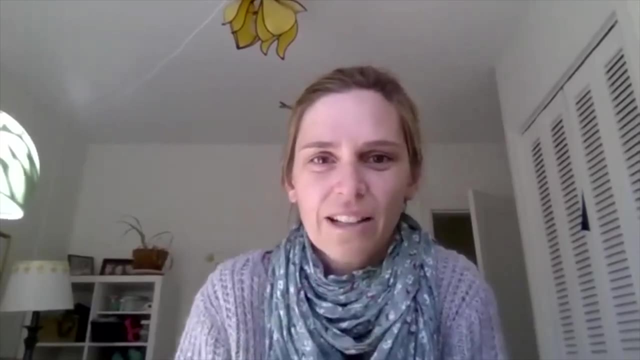 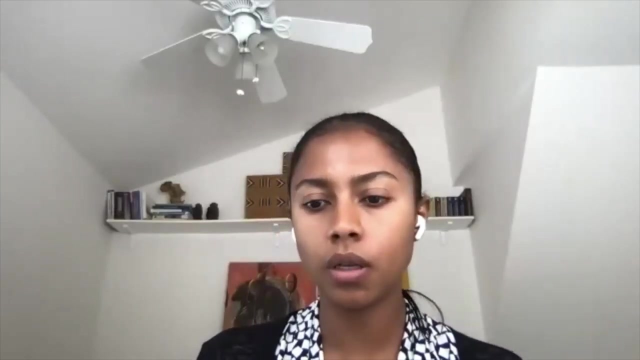 but is uh methylmercury also ph dependent and do you incorporate that into your modeling of emissions and um the way it reacts in in tissues carries up? so yeah, so yes and no, so we. the the ph question is interesting because i don't think it comes up in terms of 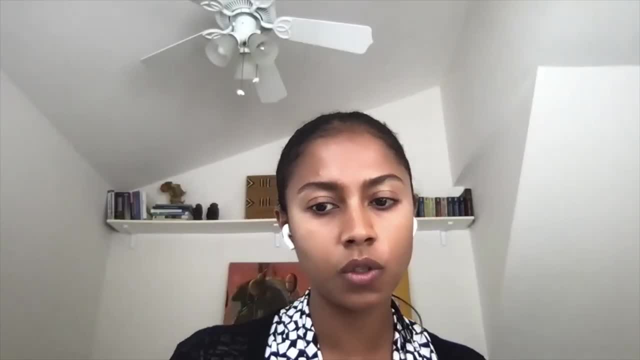 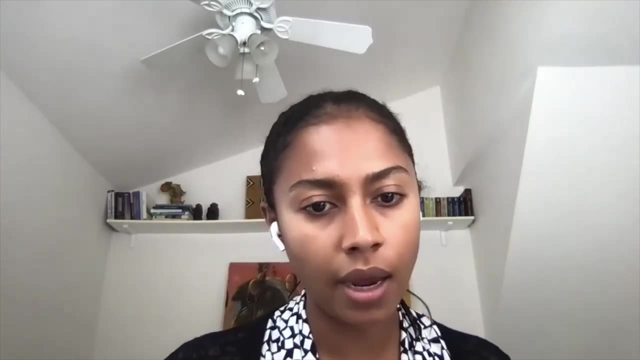 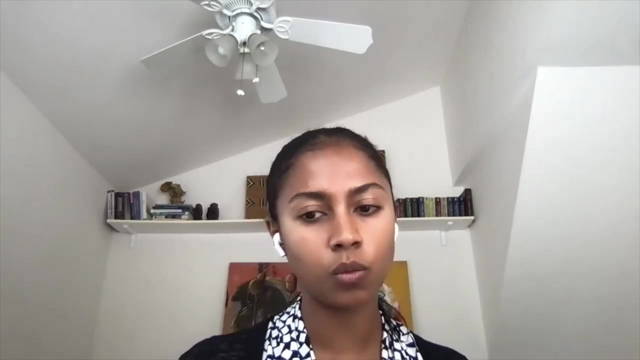 um, at least to my knowledge, i don't think that it comes up in terms of methylmercury production in the oceans, because we we're kind of still in that narrow band of ph's in sea water. that is not, i think, drastic enough to make a difference in terms of production, although you 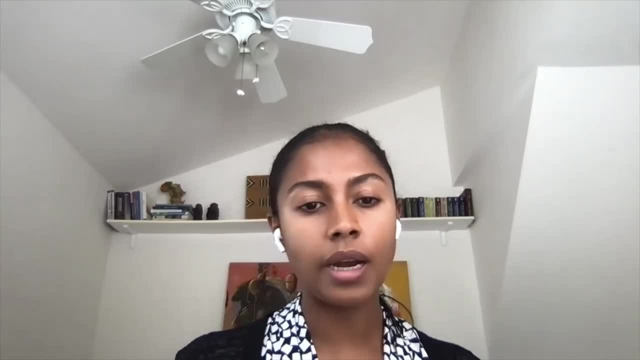 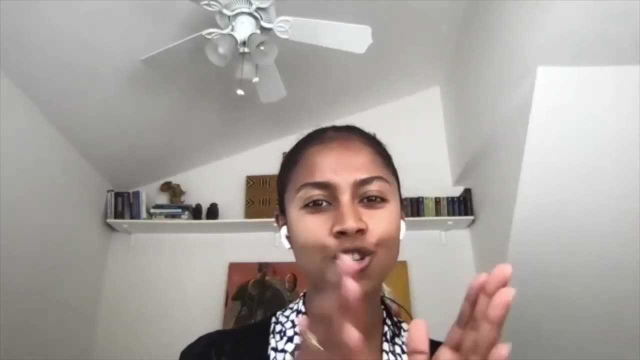 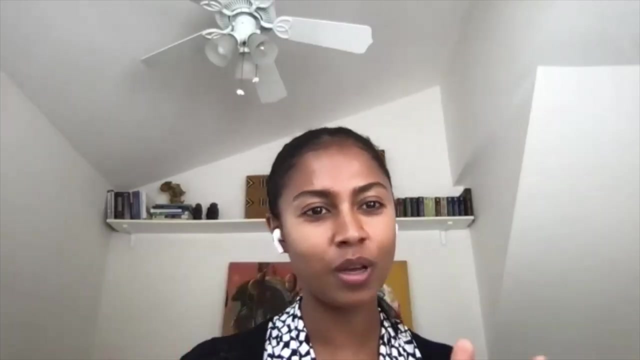 may see it if it infects the microbial communities, and i don't think that at this point we have the the capabilities to measure- measure methylmercury in such a good and repetitive way in the ocean that will capture the differences driven by a change by a 0.01 pH right? So I don't know if you see what I'm saying. 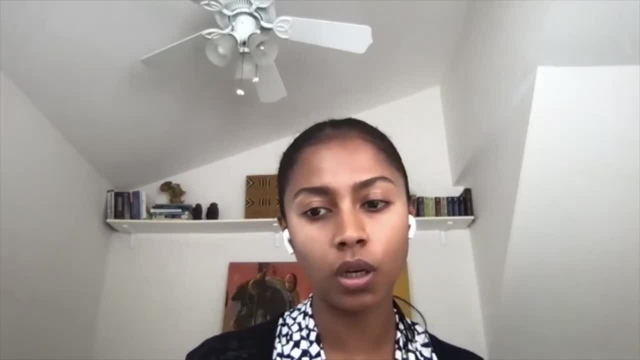 there. However, where I know that Yangshu has been working on, who is one of my collaborators, is looking at how changing pH infects phytoplankton community structure, And so if you have a change in phytoplankton community structure and methylmercury uptake is. 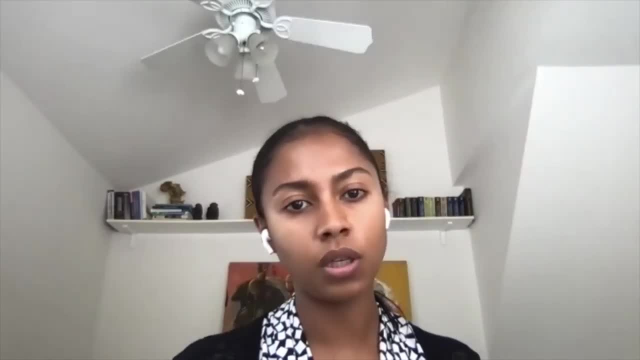 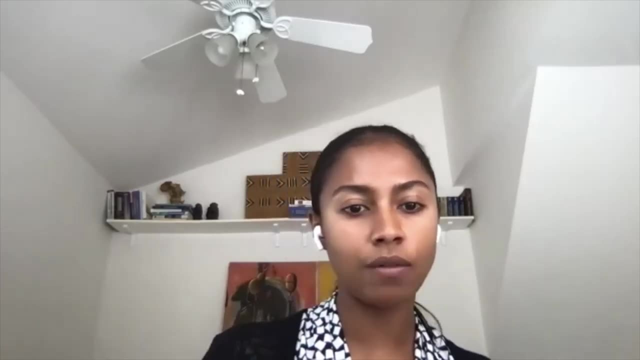 really strongly driven by the phytoplankton because that's the first step of accumulation. You go from about 10, you know the concentration- to a 10 to the 4,, 10 to the 5 increase in the phytoplankton. So if you're changing your phytoplankton community and the size of that, 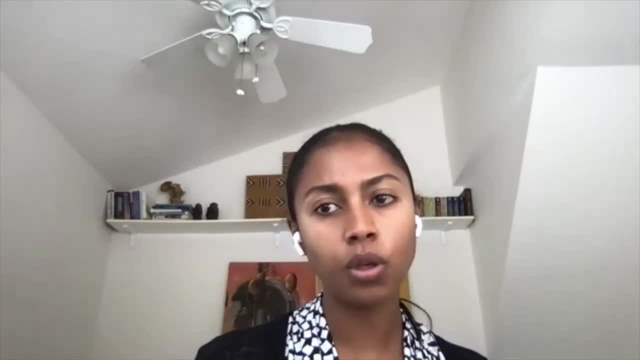 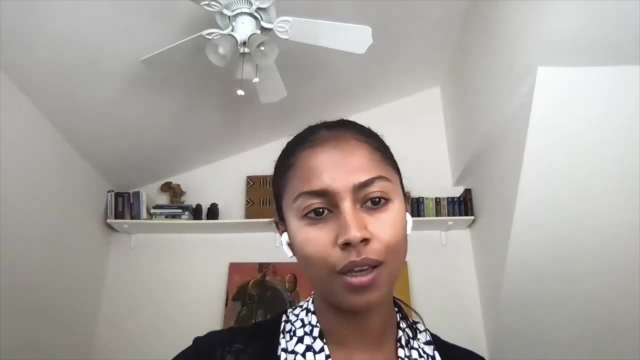 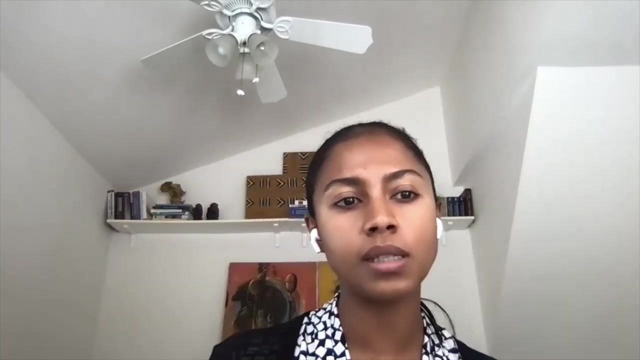 phytoplankton, you may impact methylmercury moving up, but also export, because if you have less calcifying organisms then you know you will have less export and things that don't have a ballast is not going to be exported as quickly. So I think there is some sensitivity. 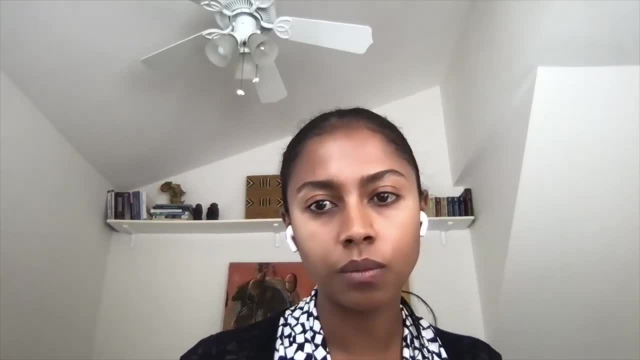 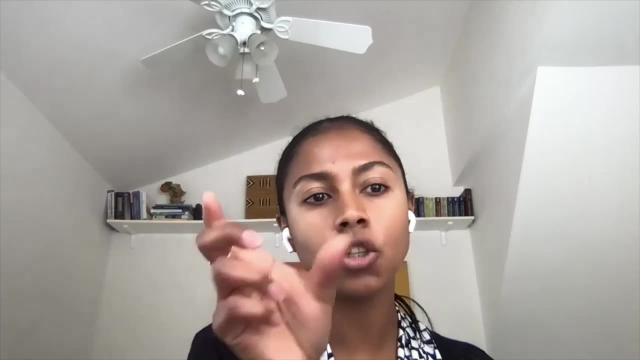 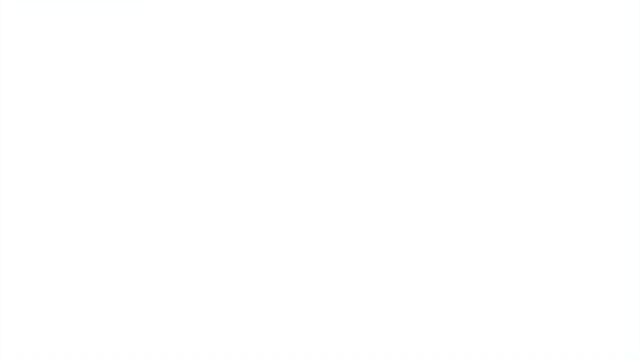 there, but not something that I think at this point is going to make a huge difference, At least in the short term. like longer term, maybe in 100 years or something like that. maybe The next question is from Anfal. Thank you for your presentation. It was very informative. I have a question: Do you face? 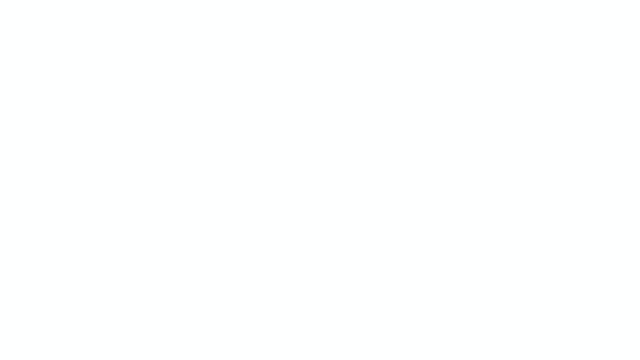 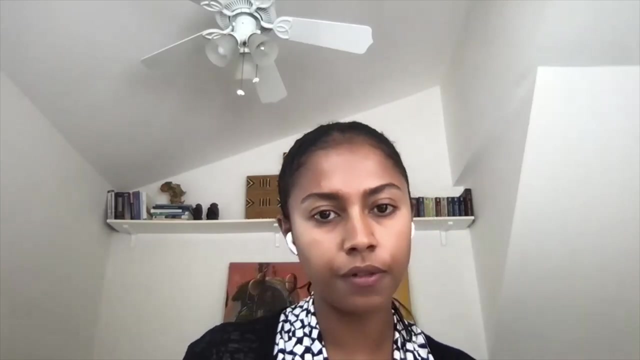 any complications Collecting data? you mentioned you took some surveys and the fishing numbers from the fishers or fishermen and you also touched up on taking hair samples And did that help. Can you briefly just talk about that? Yes, I can. I think that one thing that made a huge, huge difference and I've kind of alluded 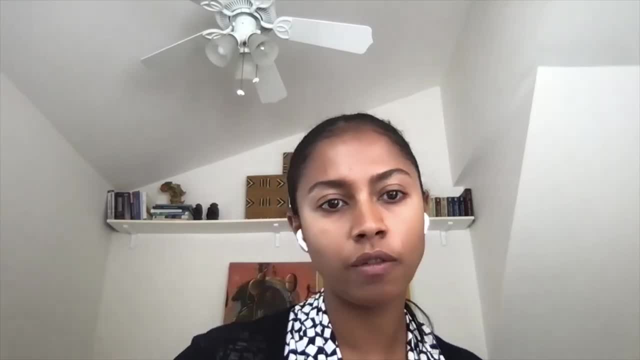 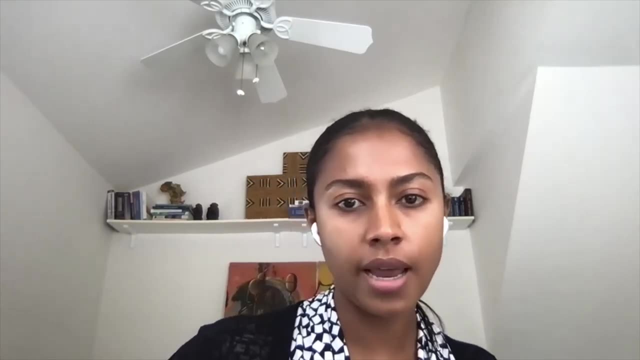 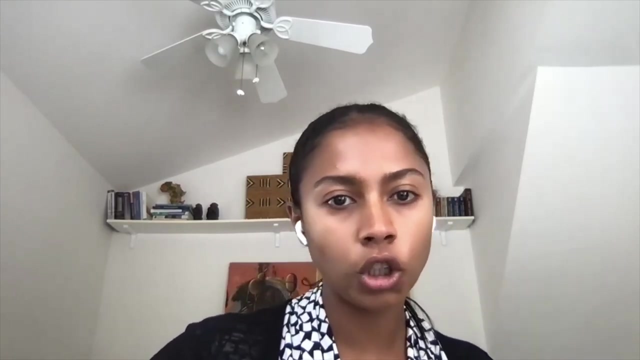 to that early on is that this was a Nazi government led Study, So they wanted to do this. They were really interested in getting the data, So they were really doing all the legwork in terms of making sure that there is like large participation. 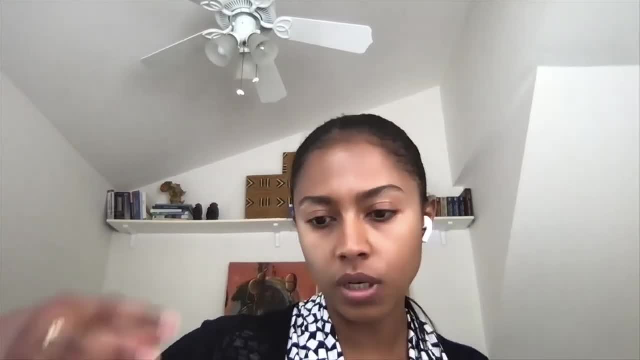 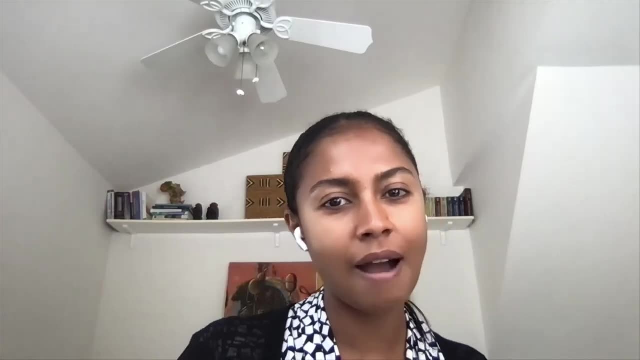 from their people, the communities that they're like, So it was really driven by them. So it made it easy for us, because we didn't have to do all the legwork in making sure that we are communicating while we're doing what we're doing. That was all done by them, And so I think that's a really good. 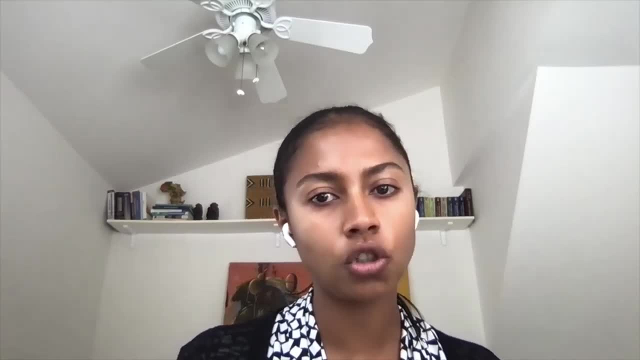 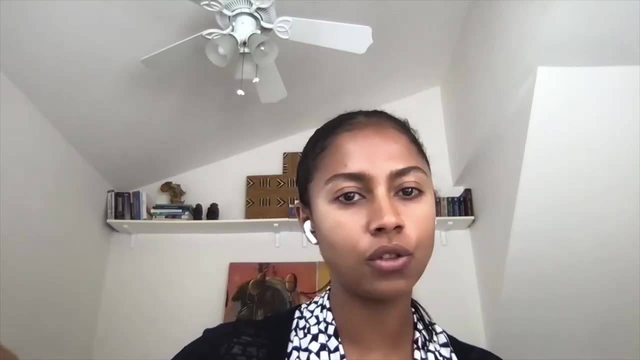 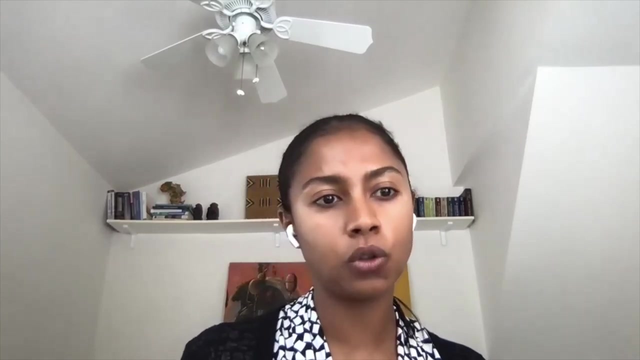 thing, And that's the government and their research. It wasn't like research, but their environmental health, environmental science staff Right. So I don't think this is something that I would be able to do by just going and knocking on somebody's door and be like 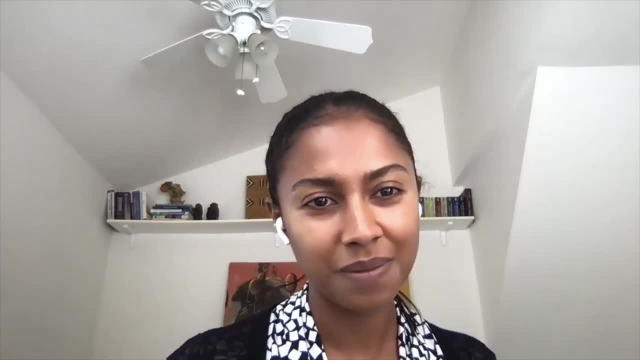 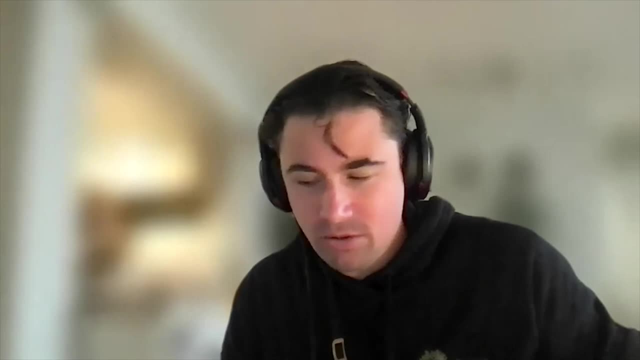 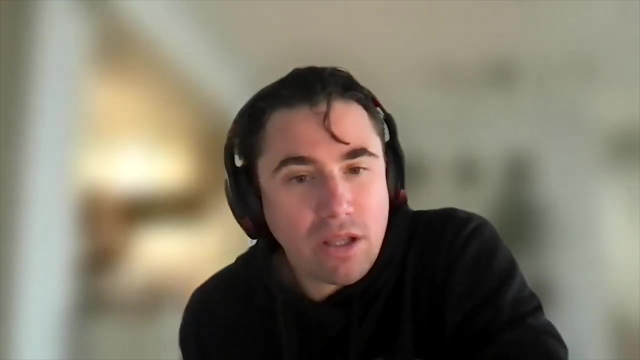 can I take your hair sample? Thank you for this answer. I had a small question: When you were analyzing the IPCC models and the scenario, did you analyze different type of emission scenario on the impact of mercury And what was the result- the different outcome of the different scenario? 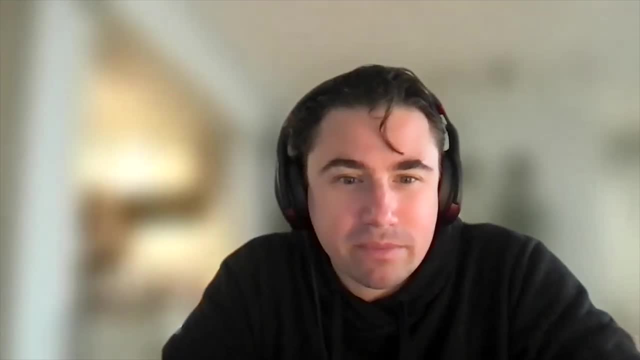 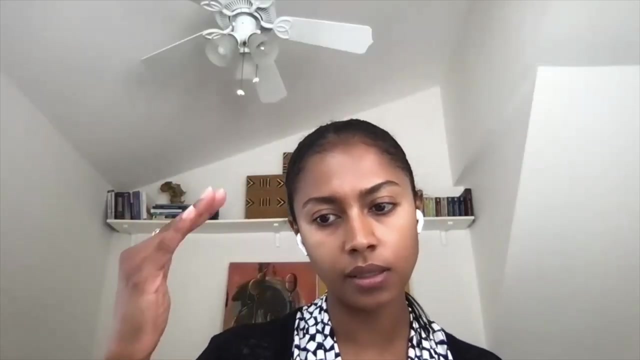 per CMIP model. Yeah, So are you talking specifically to that emissions? Yeah, I did not do that, So that was from Noel's group. Okay, So, so that was Noel and Helen That did the analysis for the different emission scenario with the models, And then we- I was on- 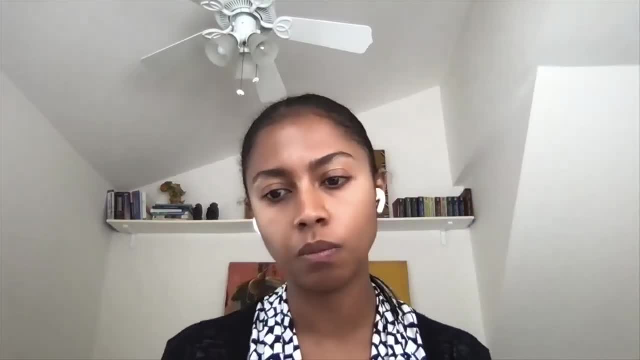 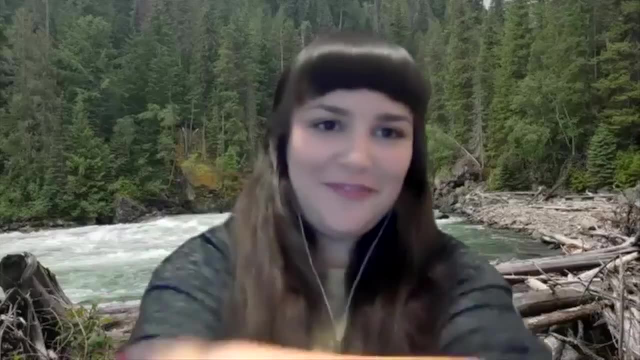 the oceans modeling team. So they provided us with the, with the, with the data. So I'm not sure how they, how they do that. I know this is also coming from another student who just was going to save it for later, but I think it's important to address the big group. Did you work with community to 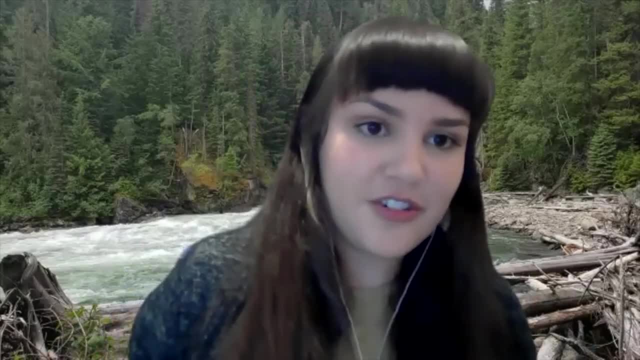 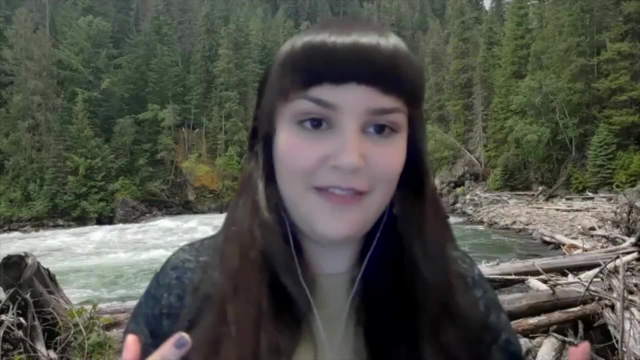 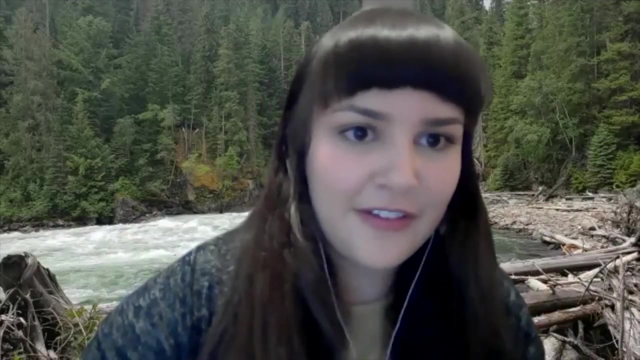 co-develop an agreement or understanding for the storage and destruction of the biological samples, Given you know that indigenous communities have traditionally had misused biological samples that have led to numerous human rights cases. Was that something that you were thinking of? Yes, I'm thinking about it. So the reason so okay, So backing up at this specific project, So, 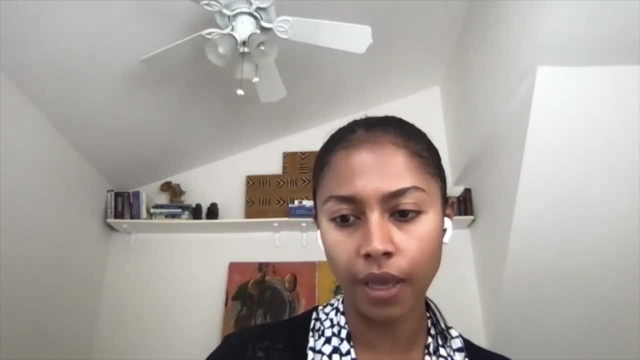 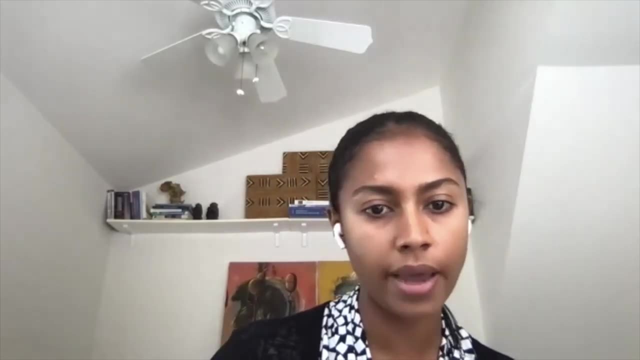 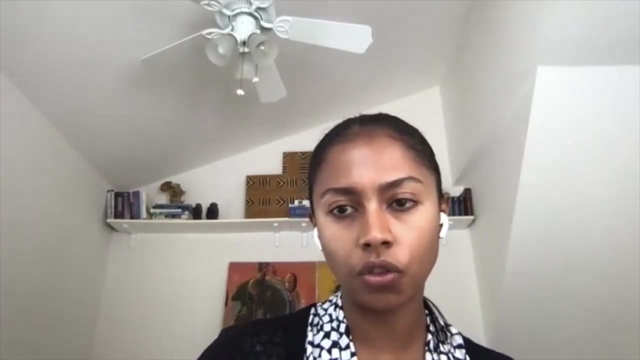 that part. so the collection of hair samples, as well as the analysis that was done by my collaborators, Ryan Calder and I think Malin Lee was involved in that. So they are. I'm not familiar, So there was an IRB process that you have to go through Harvard to make sure that all of these aspects are covered. 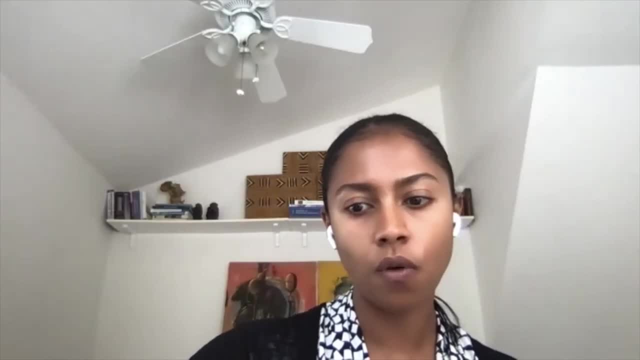 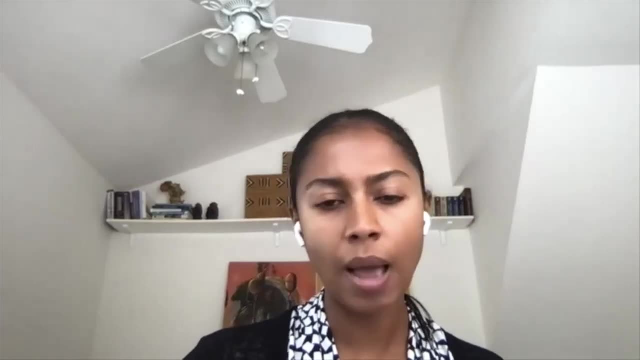 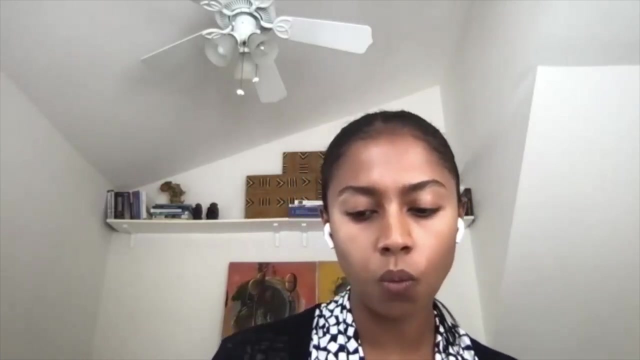 I'm not sure as to the specific details of of what they agreed with in the national government in terms of sample preservation, but I'm happy to find out And I'm I'm sure that they followed protocols Um the the I I am aware of of this and, uh, sensitive to that. So one of the things that I did, 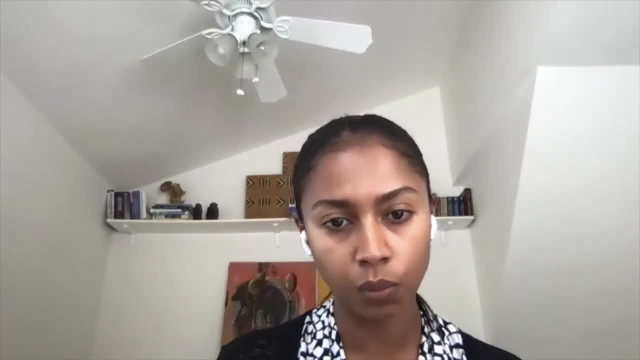 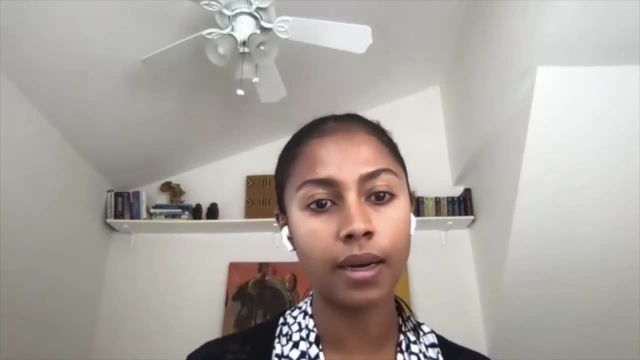 when I was in in the office of FOA programs is writing the principles for um- ethical research in the Arctic, And that was like one of the main points of that is: you know who wants the data data preservation. make sure that this remains within the communities, that they have full control. 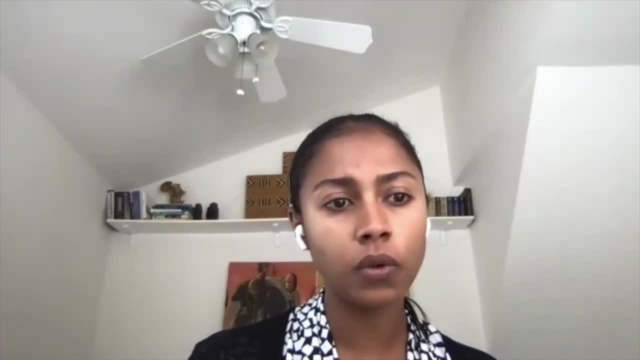 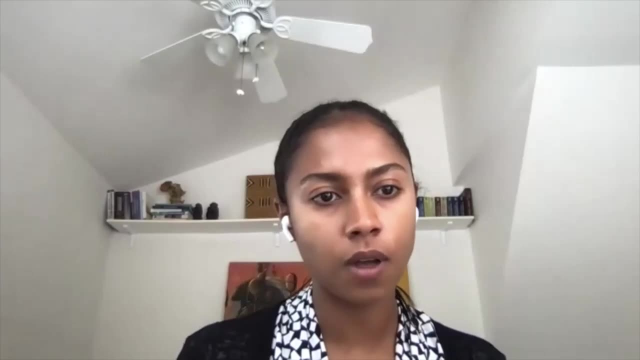 of their um biological samples, and the reasons For that are the ones that you mentioned, which were there's like a long history of misuse and abuse of uh samples that have been provided, And that's also one of the reasons why I'm very hesitant. 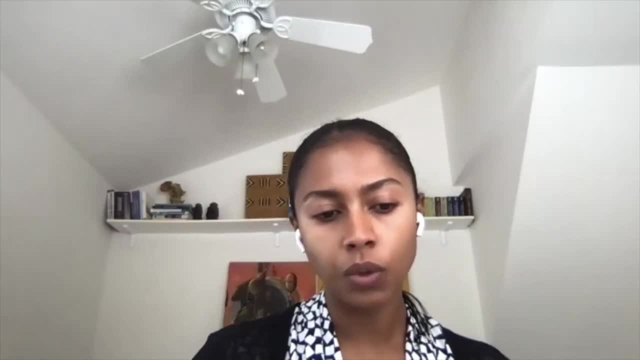 And sometimes like I'm not. I I've been really thinking about this for a long time. in a lot of I'm only interested in a one way thing, Like I'm happy if people come to me and say: we want to do this. 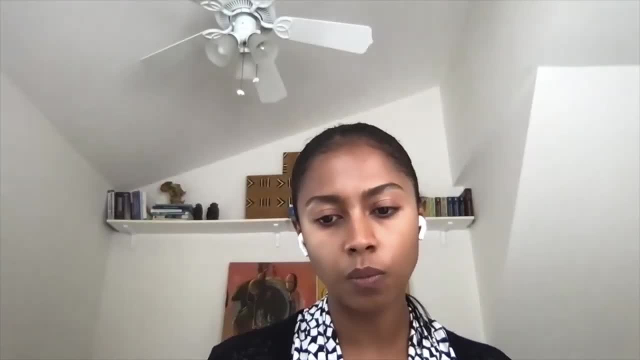 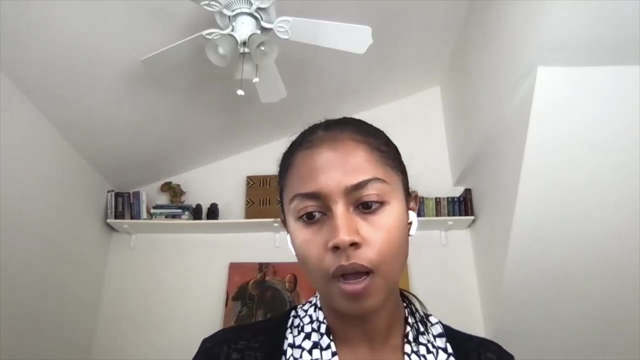 research, just what we're interested in. I'm less concerned. I'm I'm less interested in reaching out to people And say I want to do the research because of these interests, because I think that they should be coming and be driven by the communities themselves. and what are their interests? are, Um, so yes, this is a really